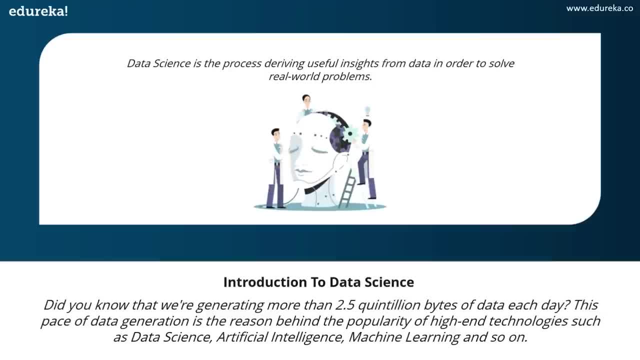 and at this pace it's only going to grow because right now, everything runs on data. So the idea behind data science is to take up all this data and, you know, derive useful insights or derive knowledgeable insights from this data so that you can grow your business or you can solve a problem. 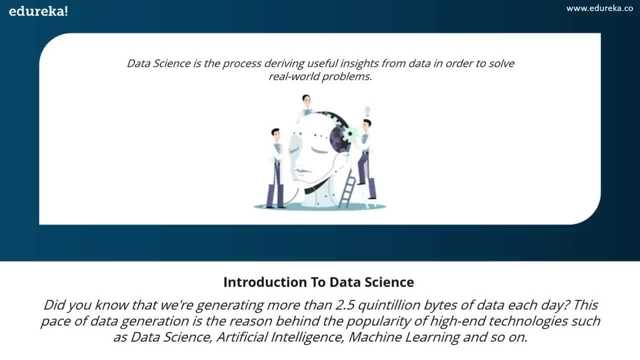 That's what data science is all about. The data is the key in data science and since we are producing so much data, it's the perfect time for you to learn data science. and data science basically covers artificial intelligence, machine learning, natural language processing. 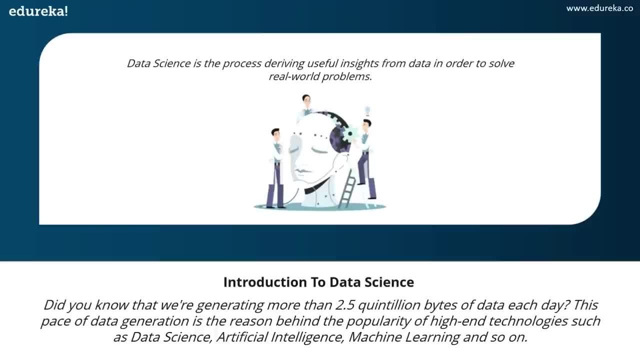 all of these processes are covered under data science, So that is one of the reasons why data science has become so popular: because of the amount of data we're generating, We need methods and technologies that can handle so much data, and they can, you know, derive something useful from the data. 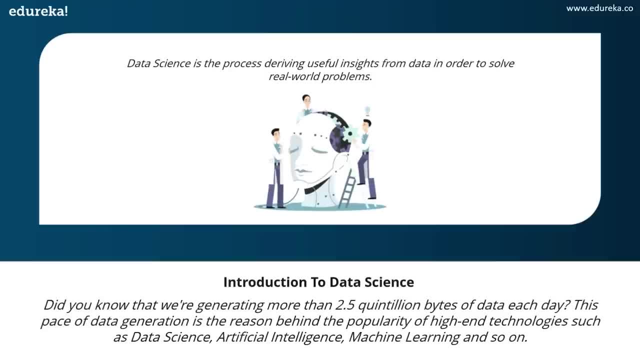 So that's a small introduction to data science, and if you guys want to learn more about data science, I'll leave a couple of links in the description box. Now let's move ahead to our topic of discussion. First, we'll understand why we need SQL for data science. 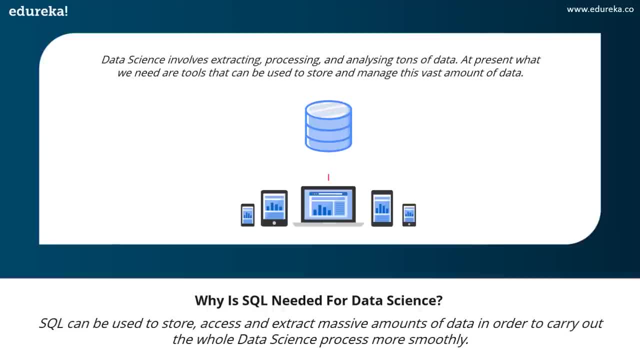 So, like I said, data science is basically all about deriving useful insights from data. Data science involves extracting, processing and analyzing tons and tons of data. At present, what we need are tools that can be used to store and manage this vast amount of data. 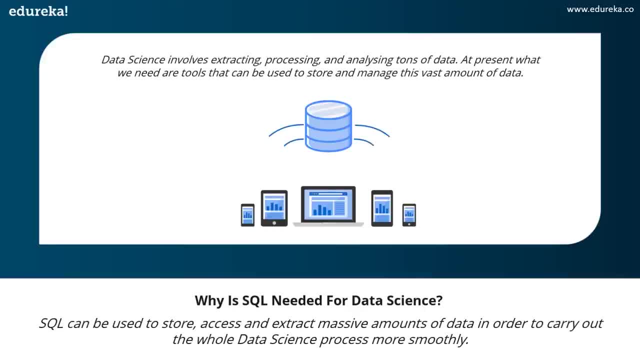 Now this is where SQL comes in. SQL can be used to store data. It can be used to access and extract massive amounts of data in order to carry out the whole data science process more smoothly. So, SQL as a querying language, it can be used to perform a lot of querying operations. 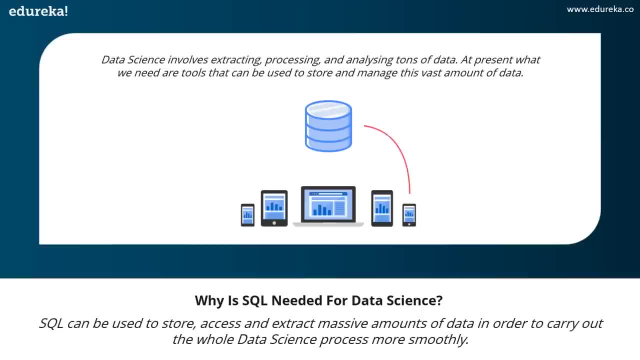 a lot of search operations, extractions and editing and modifying your data. So we need a huge management system and, along with that, we need a language that can perform all the operations that we want to do on our data. That's where SQL comes in. 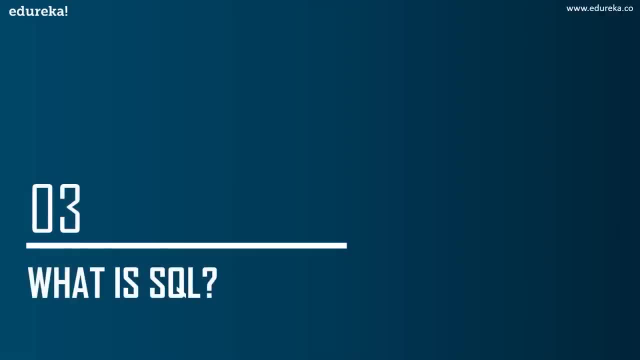 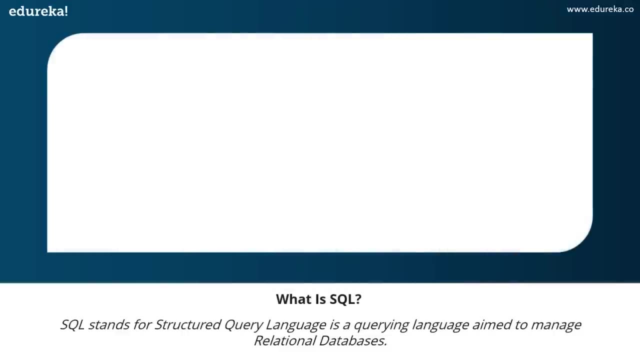 And now let's move on and understand what exactly SQL is Now. SQL, first of all, stands for structured query language, which is a querying language aimed to manage relational databases. But what exactly is a relational database, Guys? I'm just going to go through the basics here. 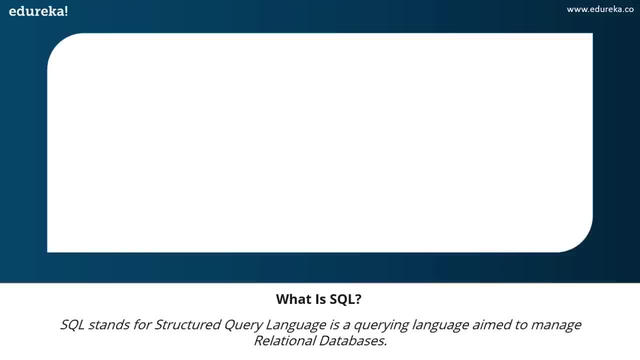 because I'm assuming that you have a good idea about SQL, because this is a more advanced topic, which is SQL for data science specifically, And so I'll just brush up a couple of things about SQL, The basic commands and a few other topics, and then we'll move on to our interesting demo session. 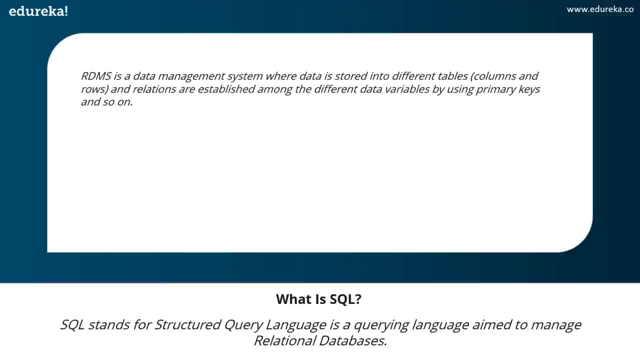 So what exactly is a relational database? Now, a relational database is a group of well-defined tables from which data can be accessed, or it can be edited and updated. You don't have to alter the database tables. Now, that's an important point about a relational database. 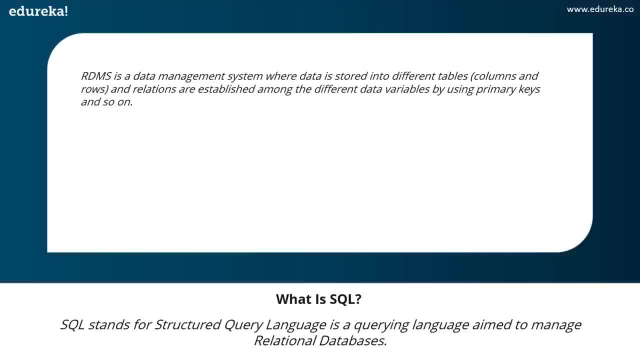 Now, SQL is a standard API for relational databases. SQL programming can be used to perform multiple actions on data, such as querying, inserting, updating, deleting, extracting and so on. So, basically, it can be used to manipulate and analyze all your data in such a way that you derive something useful from data examples. 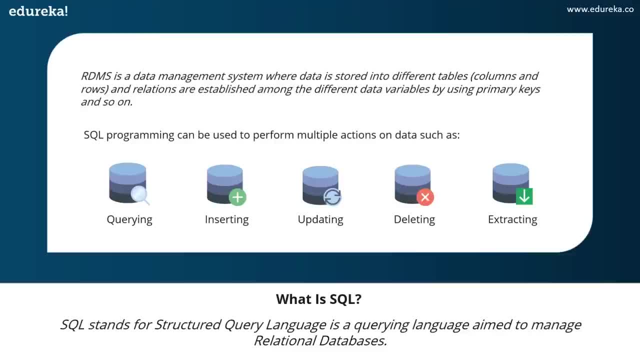 of relational database that used SQL include my SQL database, Oracle and so on. So, guys, if you want to go in depth on SQL and if you're new to SQL, then I'll leave a couple of links in the description box And you can go through those. like I said, 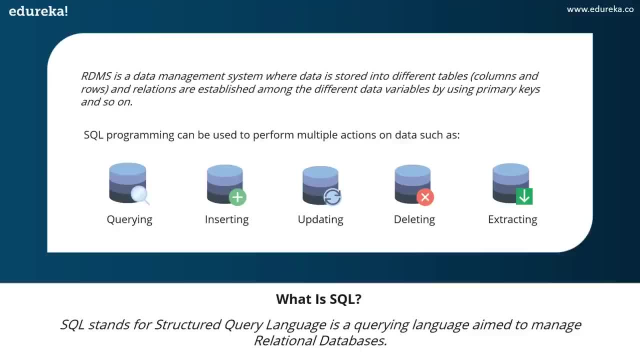 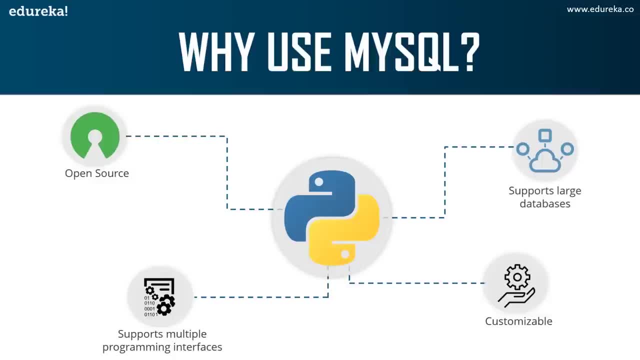 that this tutorial is mainly for SQL, for data science, and I will not be covering SQL because that is out of the scope of this session. So, like I said, we'll be using my SQL today and let's understand why I've chosen my SQL now. 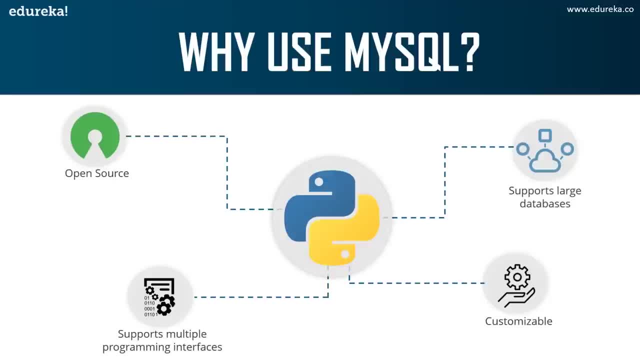 First of all, my SQL is very easy to use. you have to get only the basic knowledge of SQL right. You can build and interact with my SQL with just a few simple SQL statements. right, and SQL statements are quiet, easy, like. they're a lot like your English language. 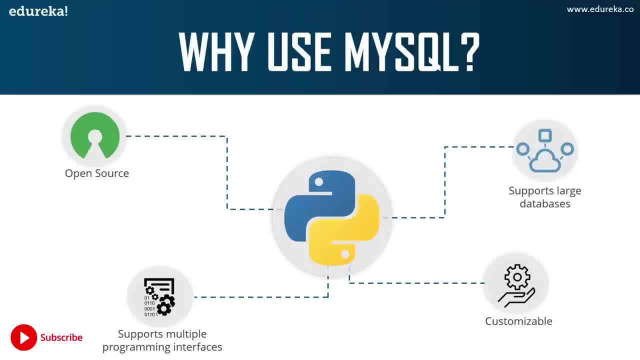 I feel like it's the most basic and the most understandable language There is- querying language. apart from this, It is also very secure. actually, my skill consists of you can see, a solid data security layer which will protect all of your sensitive data, or your confidential data, from any intruders. 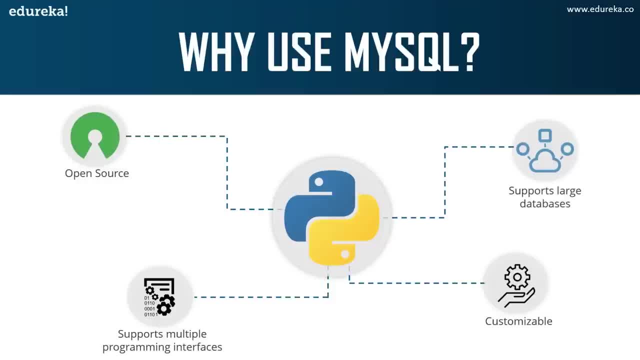 Passwords are encrypted in my SQL, So that's a good advantage of using my SQL. apart from that, of course, it's open source, So it's free to download and to use. you can just go to the official website and download it in a matter. 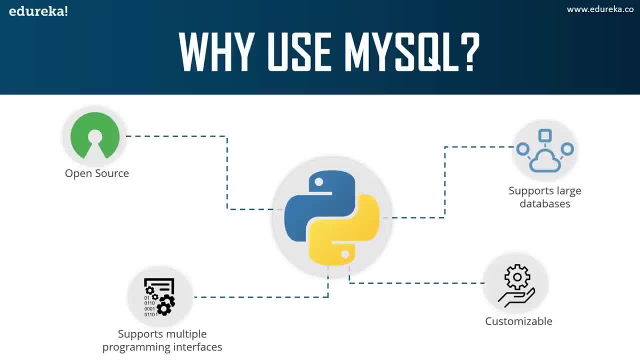 of minutes. then, of course, it is scalable as well. right, It can handle almost any amount of data. right at supports large databases up to as much as 50 million rows or more. right, That's the amount of data that you can store in my SQL. 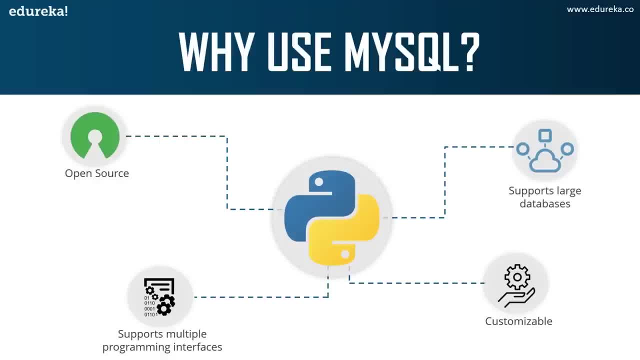 and the default size limit is about 4 GB, if I'm not wrong, and you can also increase this number to a theoretical limit of around 8 TB of data. I think you'll have to pay a little bit of money for that, But I feel like 4 GB is a lot. first of all, to have a data set. 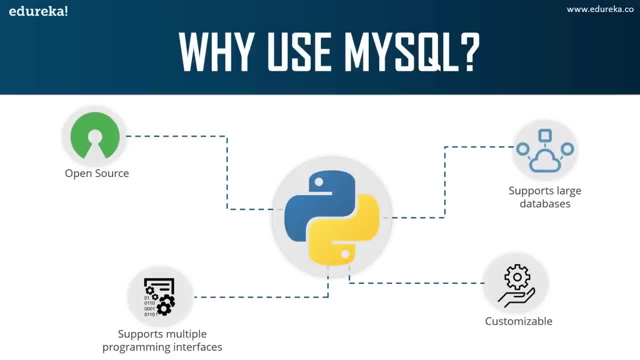 of that sites. then another important point is that my SQL follows a client server architecture, So this is where you basically have your database server, which is your my SQL, and you have many applications and programs as your clients, right, and these communicate with the server. 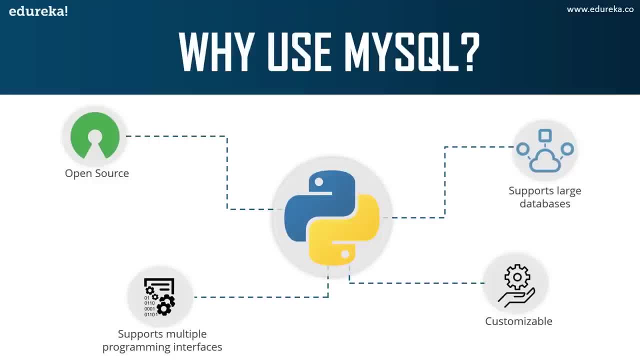 This is where they query data, They save. change is the update, the data and all of that, not only this. my skill is compatible on many operating systems. It is easy to run on a lot of operating systems, such as Windows, Linux, Unix and so on. now my SQL actually provides. 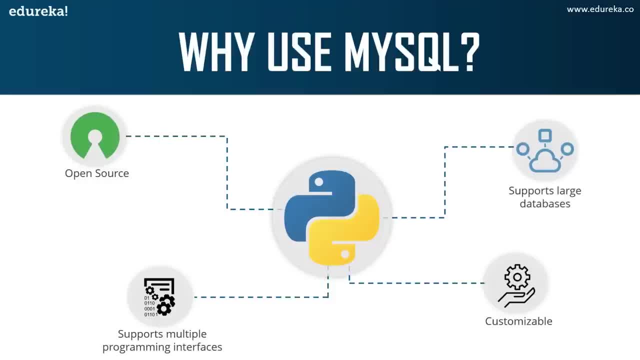 a functionality that the clients can run on the same computer as a server, or they can even run on another computer. So basically, communication via a local network or the internet. another important point is that they are quite a number of api's and libraries for the development of my SQL applications. 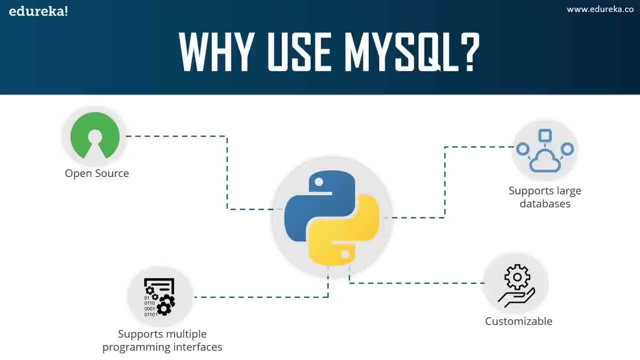 So basically, it has support for multiple programming interfaces, right? So client programming- you can use languages like C, C++, Java, Pearl, PHP, Python and so on, and all these languages are easily compatible. They provide API so that you can integrate and you can perform or you can build applications using these languages. 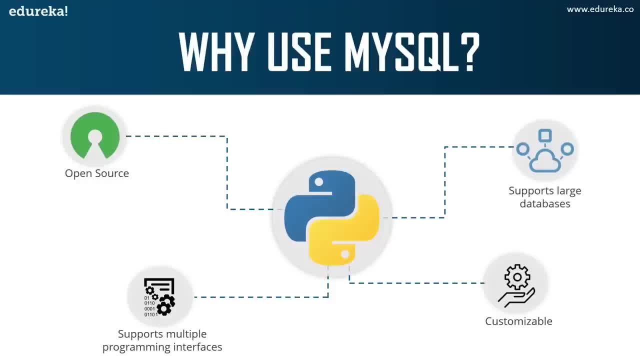 and since python is one of the best languages for data science, my SQL is Python, perfect for data analysis, storing data and querying data. You can easily work with my SQL and python to build applications and query data, and all of that right. apart from that, It is also customizable, like I said, 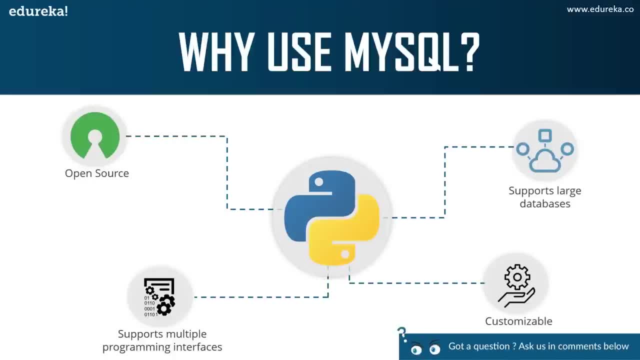 and it's also platform independent, right. It's not only your client applications that can run under a variety of operating system, but my SQL itself can be executed under a number of operating systems. The most important ones are your Mac operating systems, Linux, Microsoft Windows and so on. apart from that, 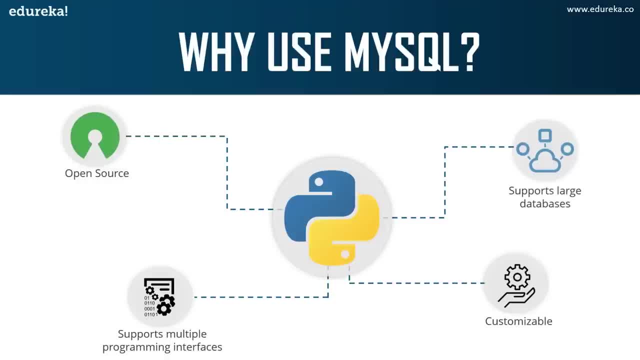 We also have speed right. my skill is considered a very fast database program and this speed is actually being backed up by a large number of benchmark tests. and apart from that, it's highly productive because it uses triggers, it uses stored procedures and views, and this basically allows the developer 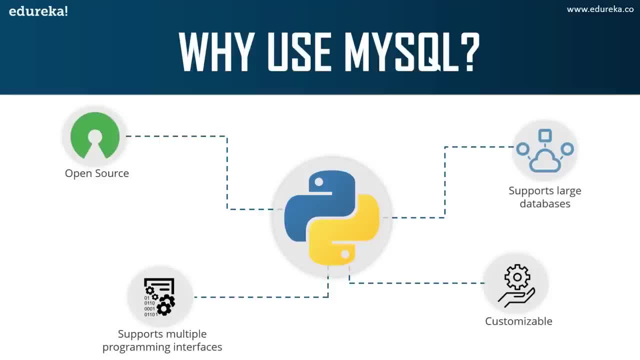 to give a higher productivity. So these are a few reasons why you should go with my SQL right. I think it's important to feel it's one of the most easiest to use and it's one of the most compatible databases that are there. Now let's move on. 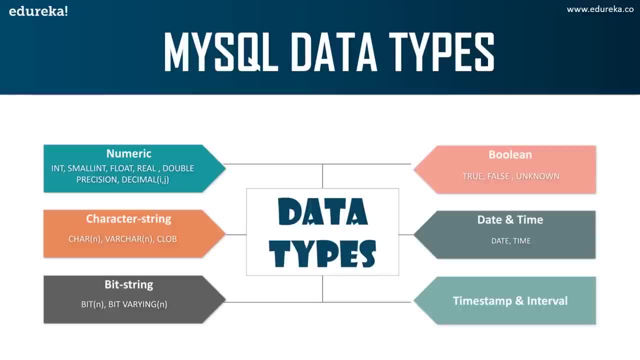 and discuss a couple of basics about my SQL. So we'll discuss the data types which come under my SQL. We have numeric, we have character string, We have bit string, Boolean, date and time and timestamp and interval it under numeric. It includes integers of various sizes. 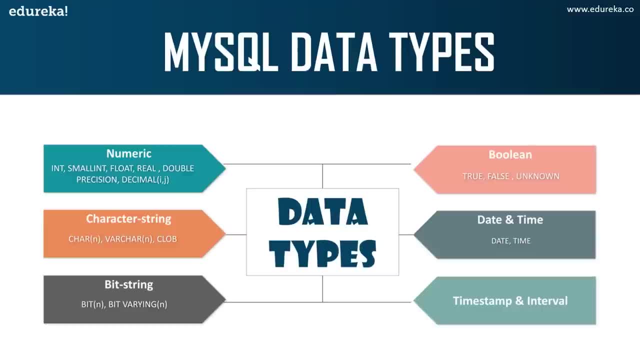 There is a floating point of various Precisions and formatted numbers under character strings. These data types either have a fixed or they have a varying number of characters. Now this data type also has a variable length string, which is called character large object, which is used to specify columns that have large text values. 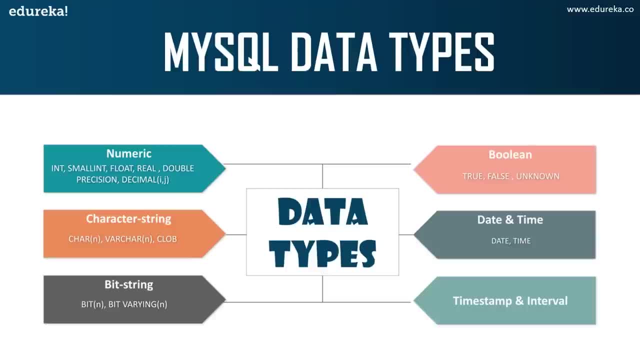 So it supports large text values as well. apart from that, there is bit string. Now these data types are either of a fixed length or varying length of bits. Now there is also a variable length bit string data type, which is called binary large object. 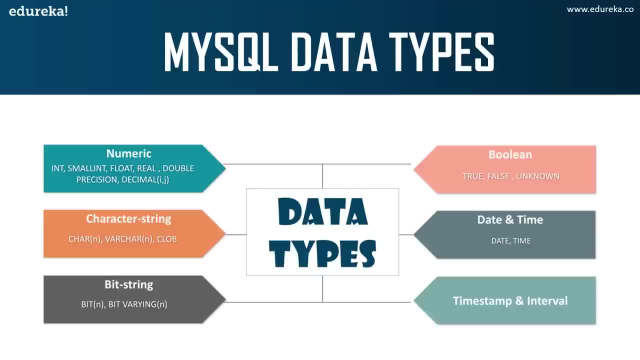 Now this is available to specify columns that have very large binary values, such, as you know, maybe images and so on. then we have the Boolean data type. Now, this data type, as the name suggests itself, It has true or false values and since SQL has null values, a three-valued logic is used. 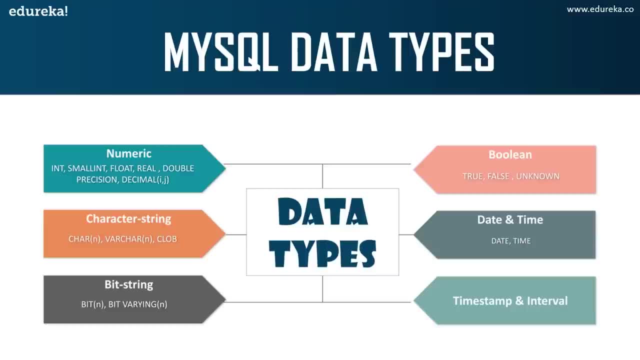 which is unknown. That's the third value. then we have date and time. So the date and time is like any other date variable. So the date data type has your month and day in the normal date form and similarly the time data type has components. 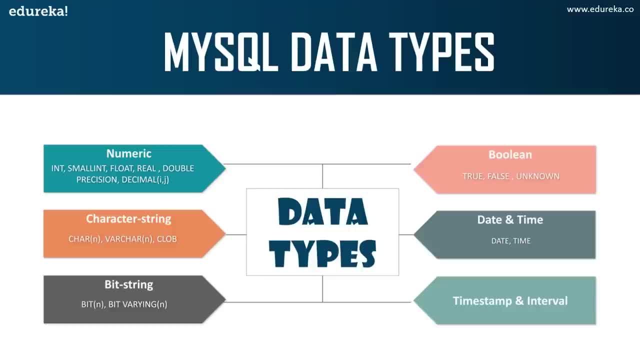 like our minute and second. now, obviously, these formats can be changed based on your requirement. next, we have the timestamp and interval data type. So the timestamp data type includes a minimum of six positions for decimal fractions of seconds and an optional with time zone qualifier. in addition, 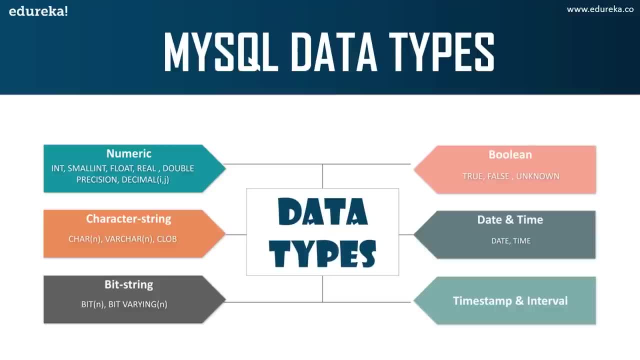 to your date and time fields. So the interval data type will basically mention a relative value that can later be used to increment or, you know, decrement an absolute value of time or date or any of that sort, or basically a timestamp. right, so you can increment or decrement any absolute value using the interval data type. 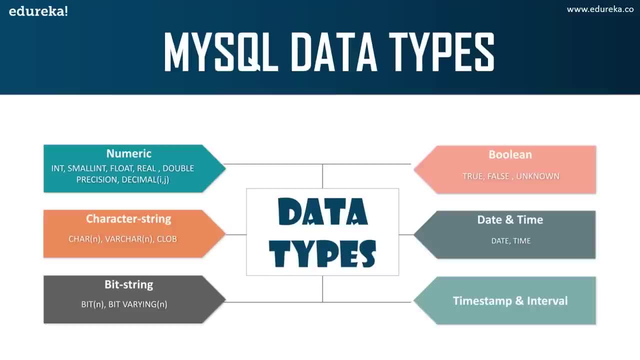 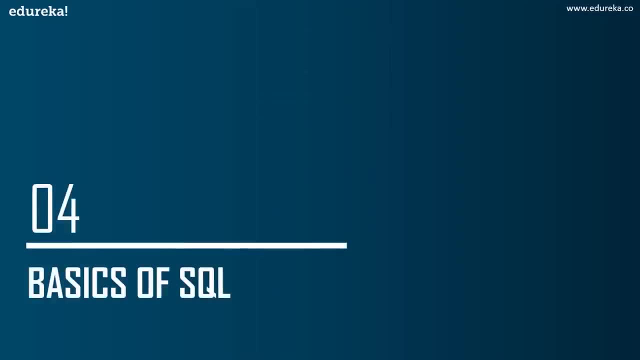 So, guys, this was a little bit information about the different data types that are there. Now let's discuss a little bit of basics of SQL. Like I said, I'm just going to brush up a couple of topics because I'm hoping that you all have. 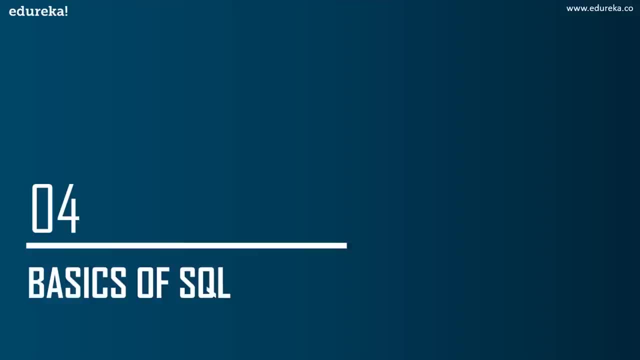 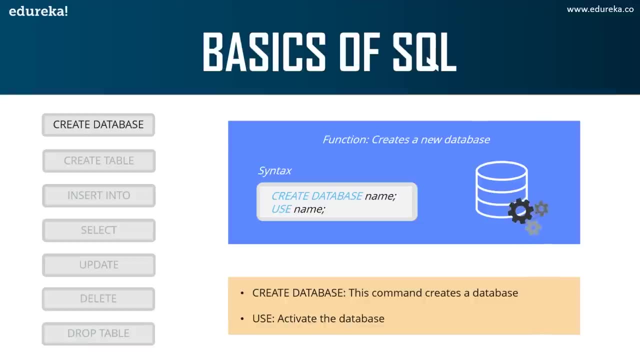 a good understanding of the querying language, So let's just brush up a little bit. So, first of all, we have the first command, which is create database, and this is a very general purpose command, right. It basically creates a new database for you. 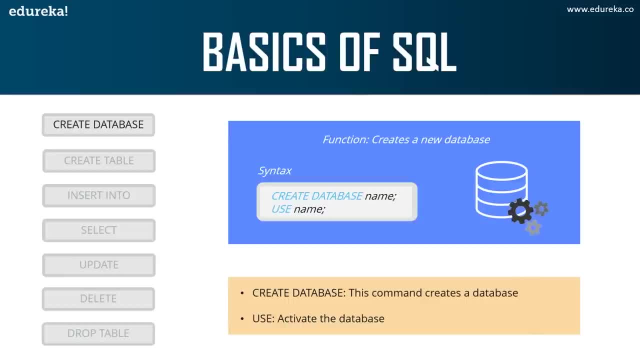 So the syntax is just create database and the name of your database. Then, once you create it, in order to initialize and use it, You just use the command use and the name of the database that you created. and remember that at the end of each command. 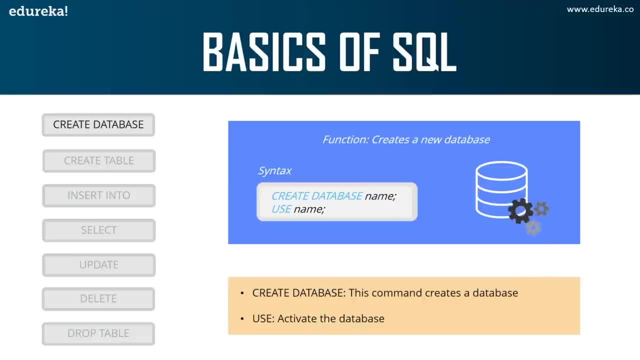 you have a terminator, which is a semicolon, and also your commands are usually written in capital letters so that you can differentiate your commands from your table columns or table names and all of that. So it's a good practice If you write all your commands in capital letters. 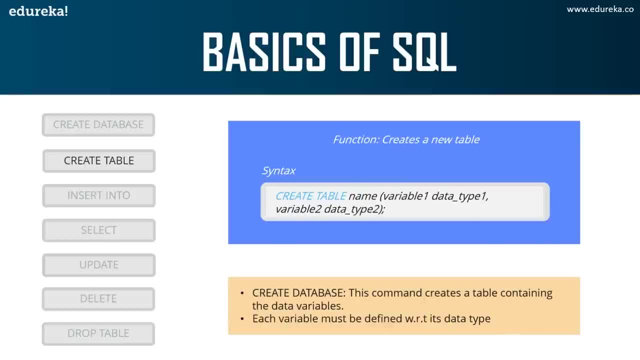 Next, we have create table. now, tables are the most important part of a database, right? so create table is a simple command that will create a new table for you, and it can contain a lot of data variables of different data types, and so the syntax is simple. 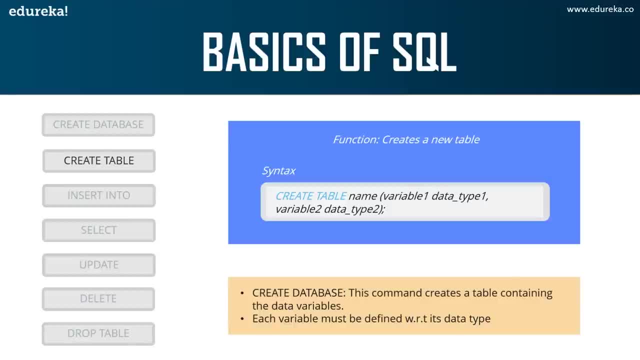 The command is create table, the name of the table you want to create, and then, within the table, whatever variables you want. You can mention the name of the variables with their respective data types, like, for example, if your variable is age, then your data type will be an integer. 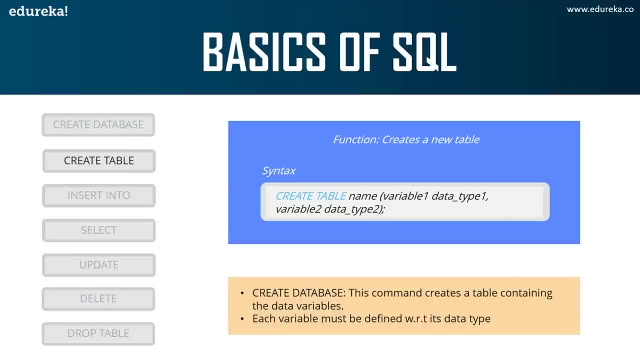 or something like that. Similarly, you can add another variable like name, and you can have the data type as a character. So it's as simple as that. It's very understandable- the language. and then let's talk about insert into. now This command is used to insert new data into your table. 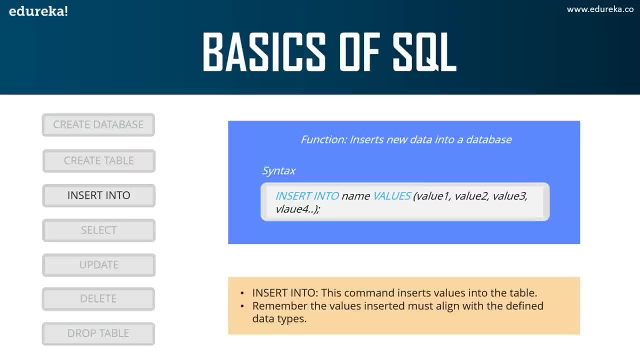 Now, usually what happens is, when people insert values into the table, they forget the data type that they've defined under that particular variable. So remember that the values that are inserted must align with the defined data types. So, for example, if your variable is age and instead. 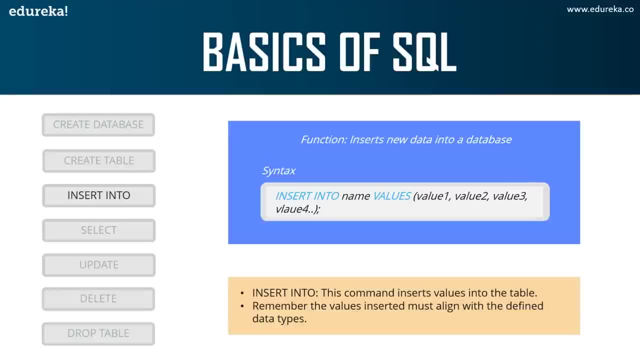 of putting your numerical three. you've put your character three Basically. you've typed out thre, and that's not going to work because you already defined your age variable as integer, So you'll get an error there. So make sure that the values that you're inserting 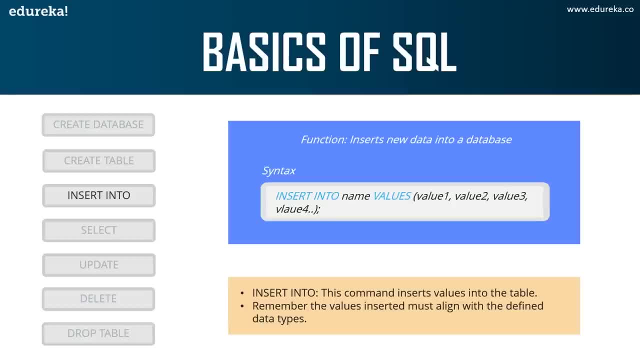 into your variable are the same data type as you've defined your variable as okay. So make sure that happens. and these are very simple things, guys. I'm sure you guys are aware of this. Now let's look at our next command, which is select. 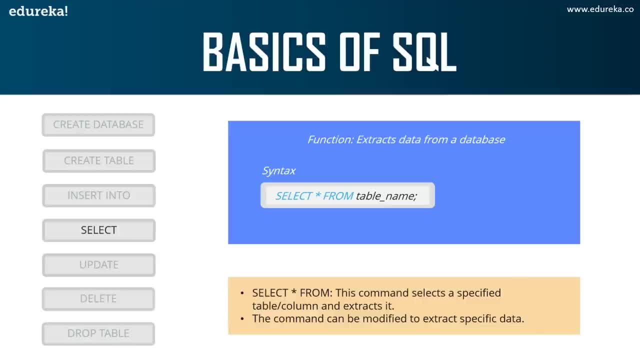 So this is one of the most important commands when it comes to SQL for data science and because mainly it's all about extracting useful insights and extracting particular type of data from your database, and we'll see how often we'll use this command when we perform our demo today. 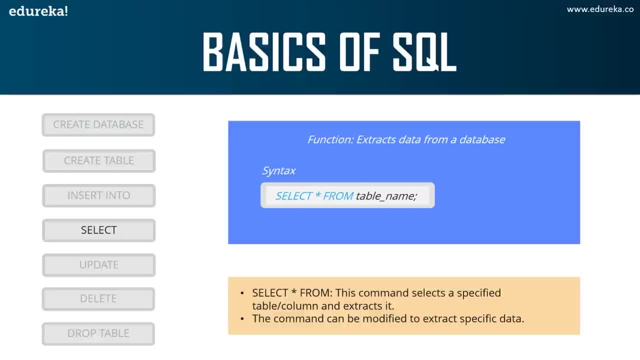 This is one of the most simplest and, in fact, it's one of the most important commands in SQL. Okay, So, basically, select will select a specified table or a column and it will extract the values from it. Okay, So select star from and table name is your syntax. 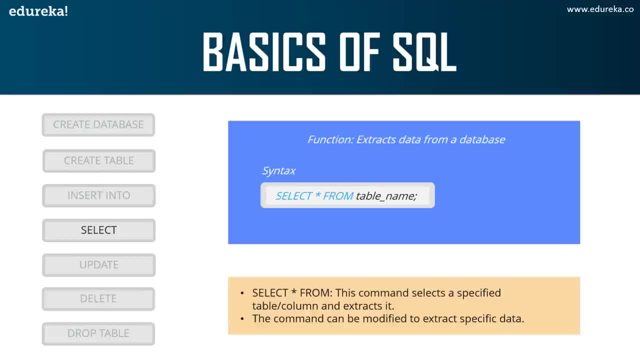 Now we'll be using this in the demo, So don't worry If you do not know exactly what this does, just remember that your select command is for extracting data from your table. Next we have the update command, So update will basically allow you to modify any values. 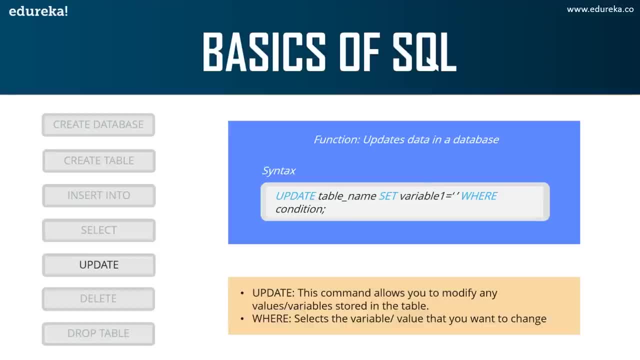 that are stored in your table, and the where clause here will select the variable or value that you want to change. So it's basically it will highlight the variable or the value, or it'll try to identify the value that you want to change. next We have the delete command. now delete. 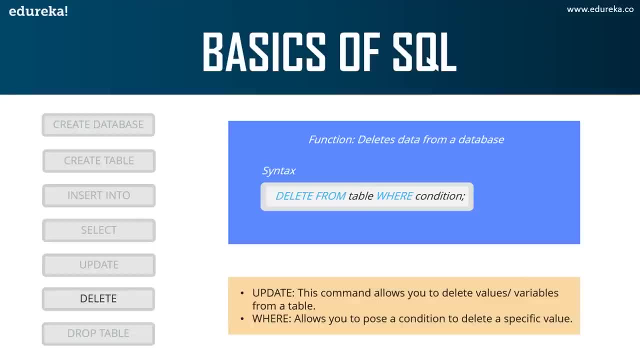 will basically delete data from your data set or from your table, as the name itself suggests. So delete from the name of your table and where with a condition. it's as simple as that. next We have a drop table, So this command is basically used to delete a table. 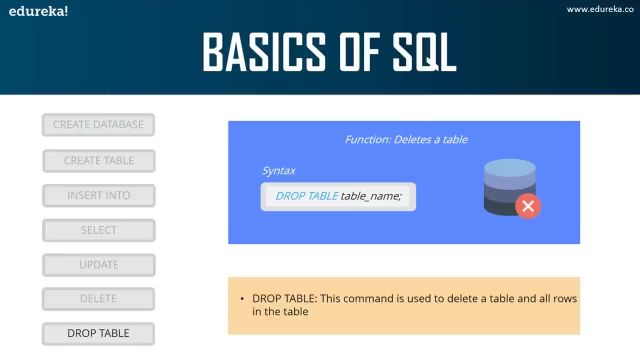 and all the rows in the table. So your table will get deleted from your database. That's what happens with drop table. These were a couple of commands that I thought you should brush up on. I'm sure you guys are already aware of these commands. 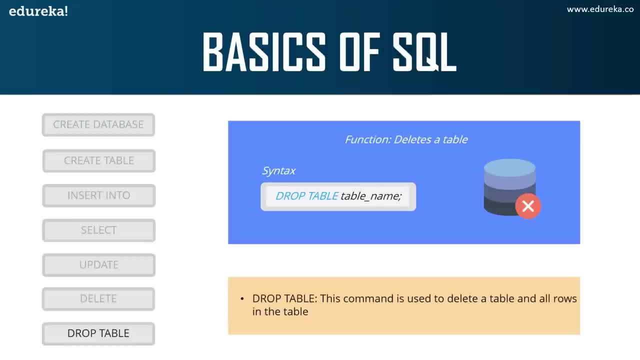 but in case there are a few of you who don't know much about SQL, I'll leave a couple of links in the description box. You can go through those videos and then maybe come back to this if you're specifically looking for SQL for data science. 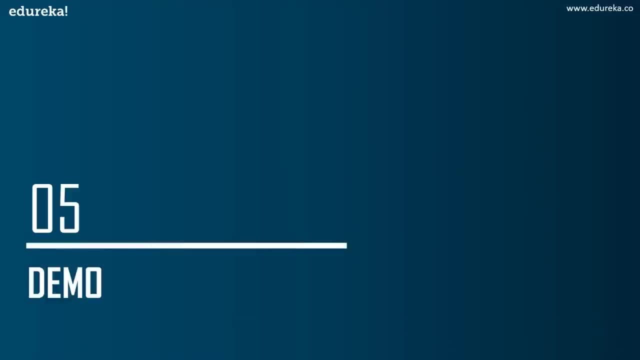 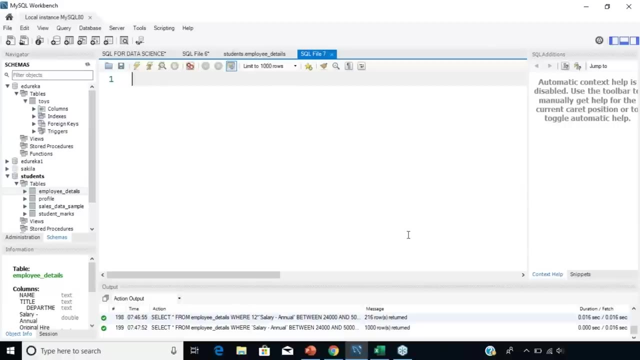 Now let's get started with our demo, which is quite interesting. So, guys, with this demo I'll be using the MySQL workbench, So it's quite easy to install. It'll just take like 15 to 20 minutes. I'll leave a link in the description box. 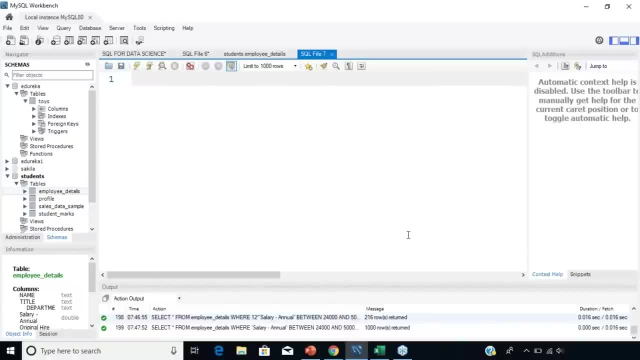 We have a short video where in me, showing you how to install the whole workbench. So once you've installed MySQL, we'll start by creating a database and we'll import a data set into our workbench. So I'm going to import a existing data set, right? 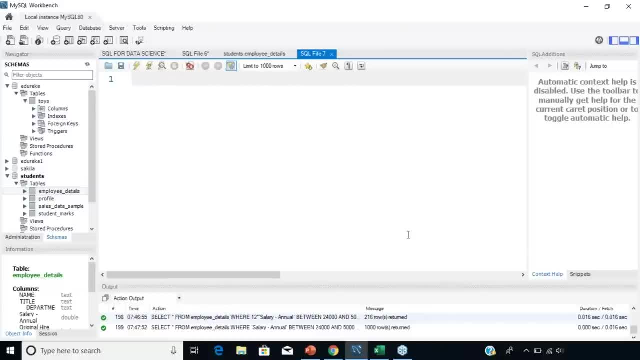 I'm doing this because we are doing a more advanced tutorial. This is not about creating tables, and you know extracting values from tables. instead, This is about deriving useful insight from your data. So usually for data science, you don't have to sit down and create tables. 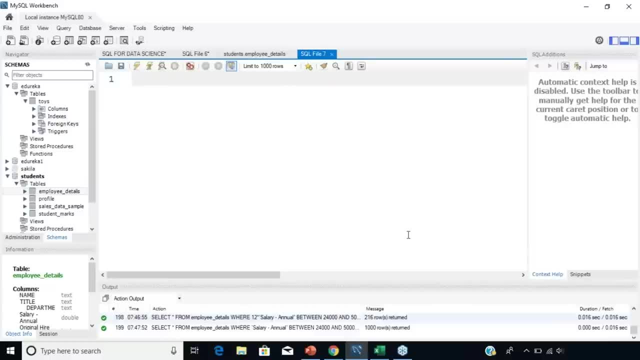 and, you know, do those basic commands. Instead, You have to explore the data variables. So usually there's a humongous data set that needs to be explored and analyzed in order to derive something useful from it. So that's what we're going to do today. 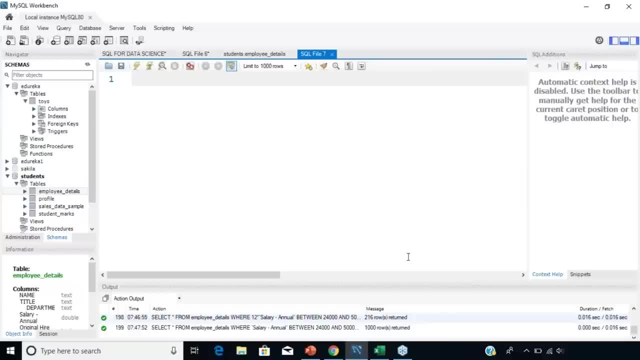 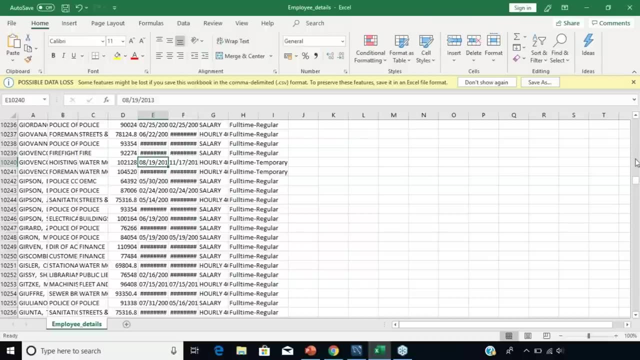 So I've already imported a CSV file. Let me show you what the file looks like. That's what this is, our CSV file, and this basically contains details about employees. So basically, the name of the employee title is the job title of the employee department. 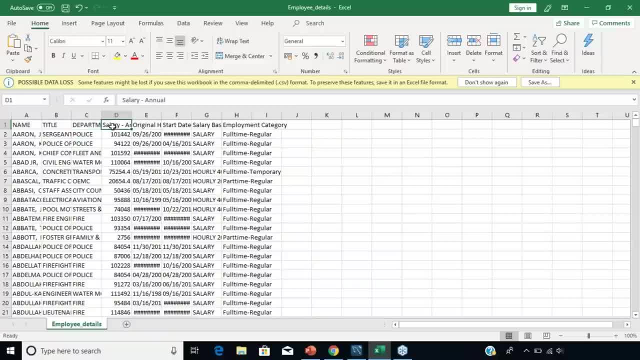 is the department that the employee is working in. then we have the animal salary, We have the hiring date, We have the start date in the present position, We have the salary and we have the employment category, whether your full-time employee or whether your part-time employee. 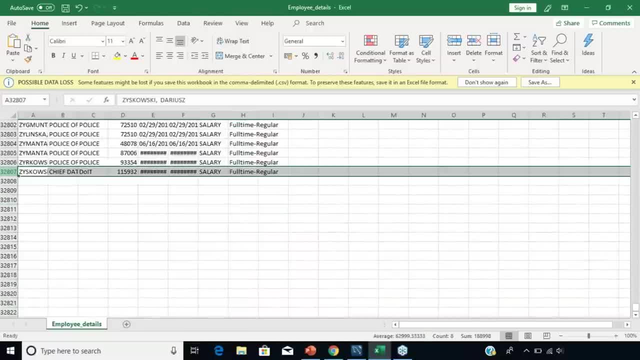 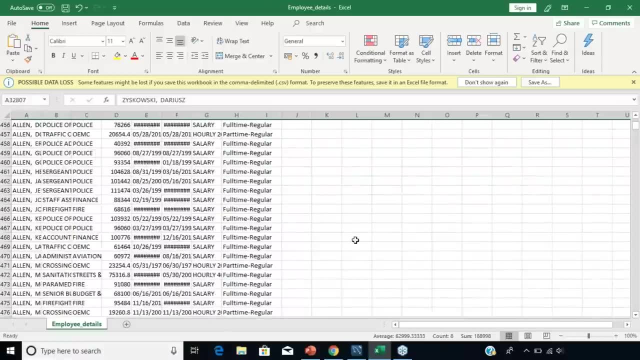 So our data set has around 32,000 observations, right, So this is a very huge data set and I basically downloaded from the internet. You can find a lot of data sets on the internet and you can perform all of the data analysis in no time. 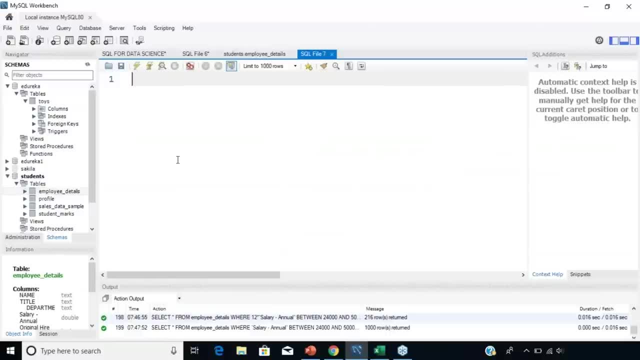 So if you don't know how to import a data set in your MySQL workbench- and I'll quickly show you how it's done- So I've already created a database here Now. creating a database is as simple as this, right, You just have to do create. 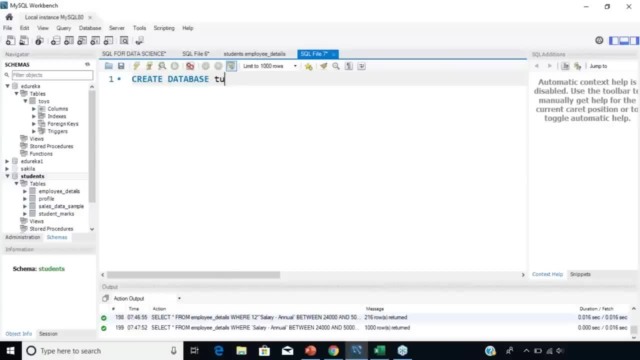 Database and name of the database, Let's say tutorial- And then if you want to use it, you just use the command use tutorial, Right, So the tutorial database gets activated. Now all you have to do to run is you have to use this. 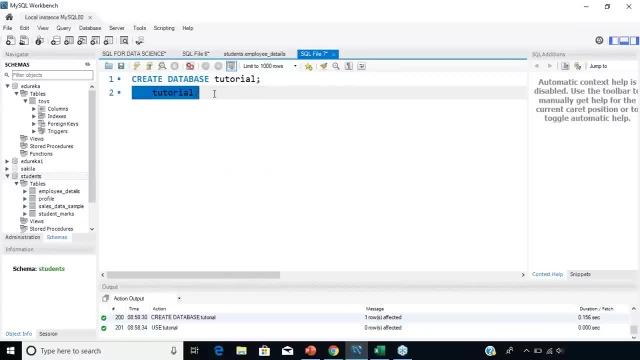 right use tutorial. So we've basically activated our database now for this tutorial. I've already created a database, So I'm going to use that database itself. Name of my database is students, And so let's activate this database right now in this. 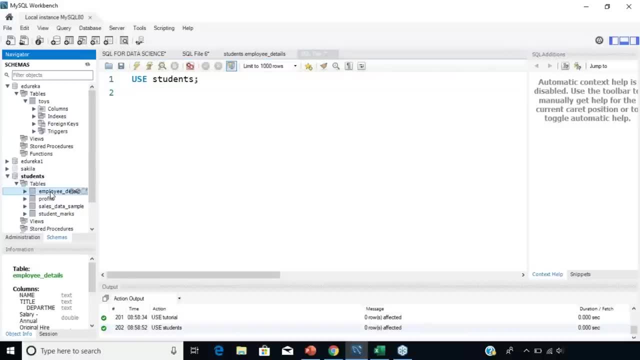 I have a couple of tables, and we are going to be focusing on this table- employee details. So this is the table that I imported. So, guys, for those of you who don't know how to import a CSV file into your MySQL workbench, All you have to do is go to tables, right click on any table. 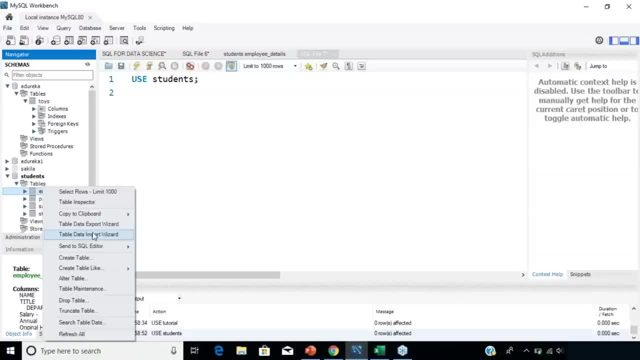 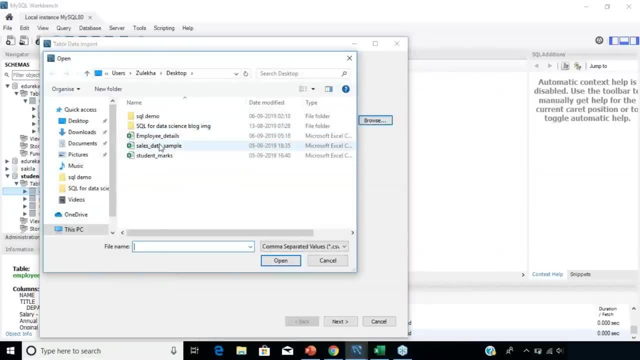 and go to table data import wizard And click on this and browse for your CSV file. Okay, just to take an example, I'll consider this CSV file. I'm not going to import the CSV file that we're going to be using right now. 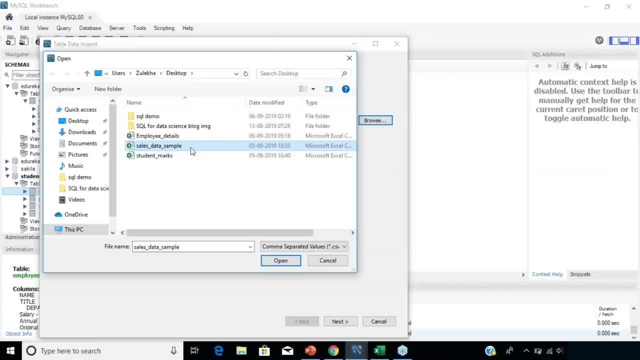 because that is a very, very huge CSV file and it'll take a lot of time for me to import that CSV file into the workbench. to save up on some time, I'll import a small CSV file and I'll show you all, and so I'm selecting this file. students marks. 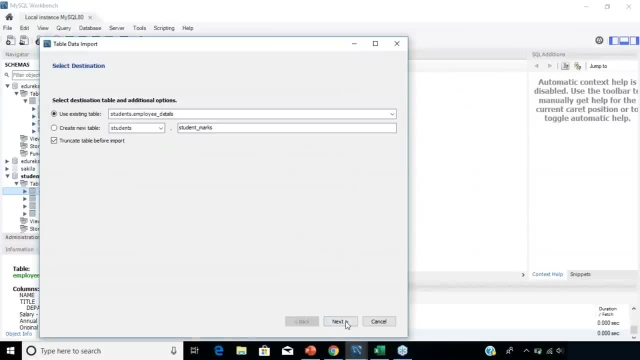 Let's open it Right and go to next. after that, create a new table. Now, basically, what you're doing here is you're going to create a new table that corresponds to all the columns that are there in your CSV file. either you can create a table on your own. 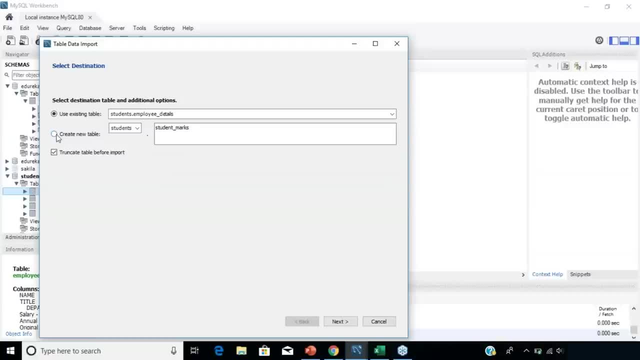 and click on use existing table, or you can allow my sequel workbench itself to create a new table for you. That's what I'm going to do, because obviously it's simpler. then click on next. So this is basically all the fields that are there. 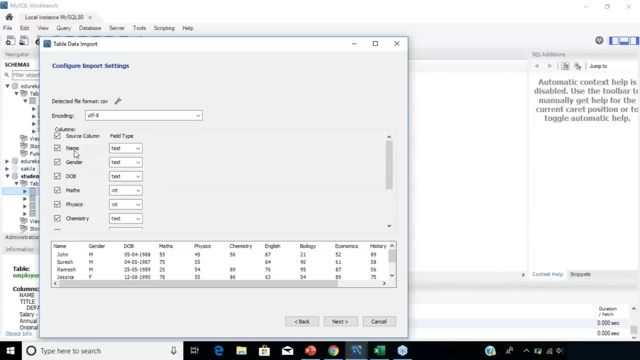 in my CSV file. It will collect all the fields in my CSV file and it will create a table out of it. right? This is my CSV file. Basically, It has name, gender, date of birth, math, physics, chemistry and all of that. These are just records of students and their marks. 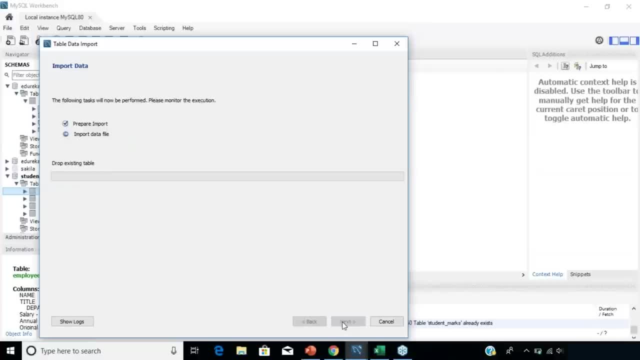 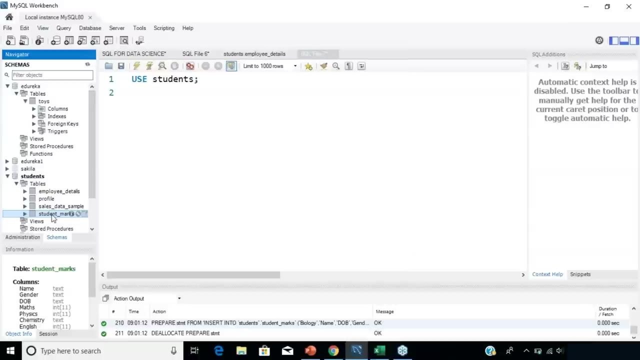 then if I click on next and next, again, Yeah, data gets imported. next five records are imported. click on finish and refresh. Here you'll see student marks. So this was the CSV file that I just imported into my sequel workbench. So, guys, that's how you import a CSV file. 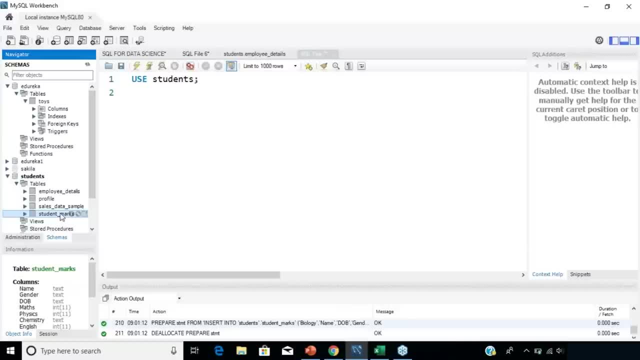 as a table into your my sequel workbench. So if you want to see this table right, the CSV file that we imported as a table- All you have to do is select, start from and the name of the table- It is student, underscore marks. 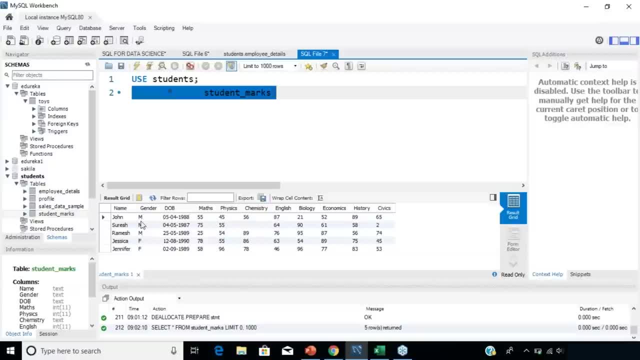 So let's just run this. So here you can basically see the entire CSV file that we imported into a table. So, guys, that's how simple it is to import a CSV file into your- my sequel- workbench in order to perform data analysis. 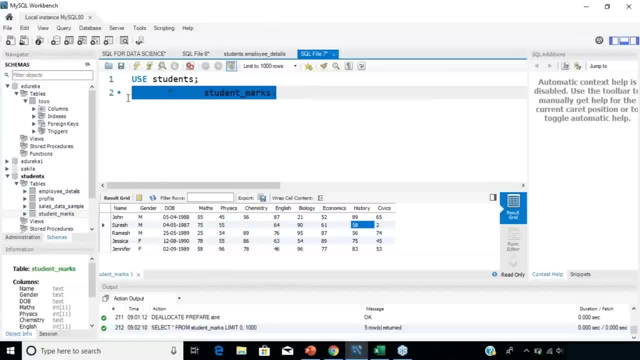 So now let's clear this up. So for this demo, like I said, we'll be using employee details data set. This is a very huge data set and let's just get started. I've already imported the data set here as a table right. 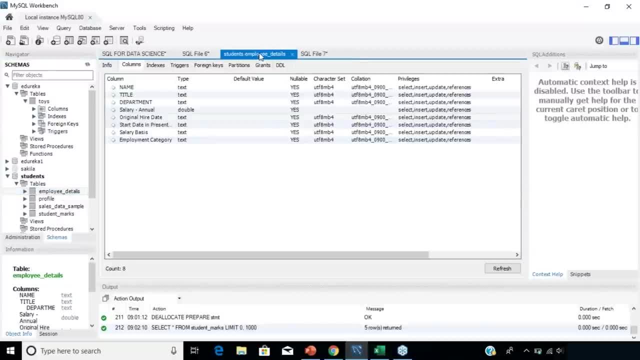 If you take a look at this: employee details. So these are the columns in my table. We have name of the employee title. is the job title of the employee Department. is the department He works in salary- annual salary. Then we have hiring date, start date, salary basics. 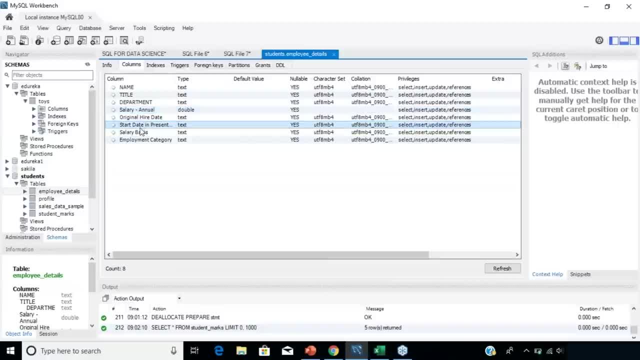 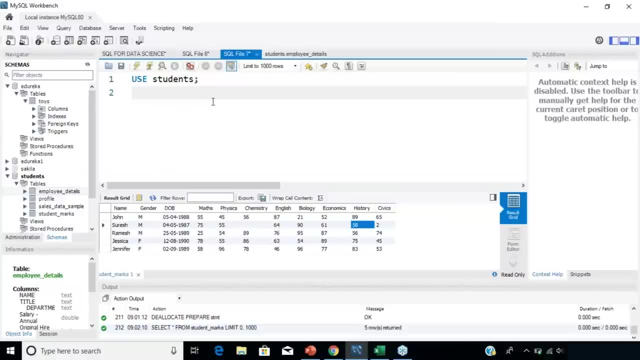 and we have employment category, All right. so let's start by performing some sort of data analysis. So first, what we'll do is: let's just take a look at the data set. So let's take a look at the data set. So let's take a look at the data set. 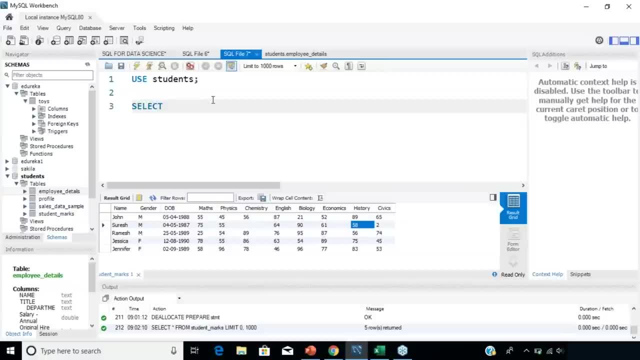 So let's take a look at the data set. View the entire table that we have. for that, All you have to do is select star from the name of the table. employee details is the name of the table in my case, So I'll just run this command. 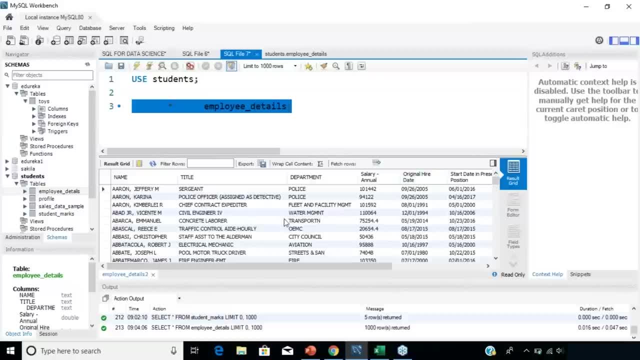 Right, So this is the entire table. that just got loaded, right? So this will just extract your entire table for you, since I did select star from and name of the table, So my entire table is extracted here, right, If you take a look at this: the whole table. 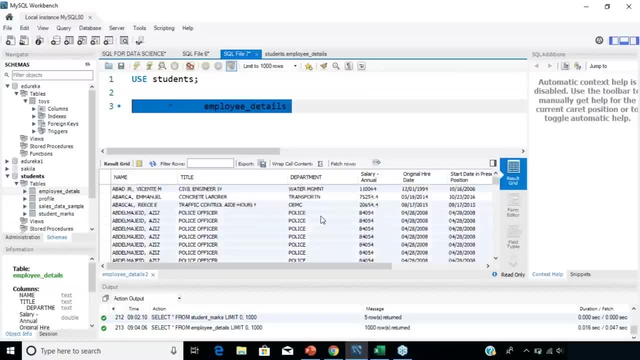 is being extracted here right Now. let's do something a little more complex. Now let's write a query to find the salaries of all the employees. for that, What you have to do is select again now name of the column that has the salary. 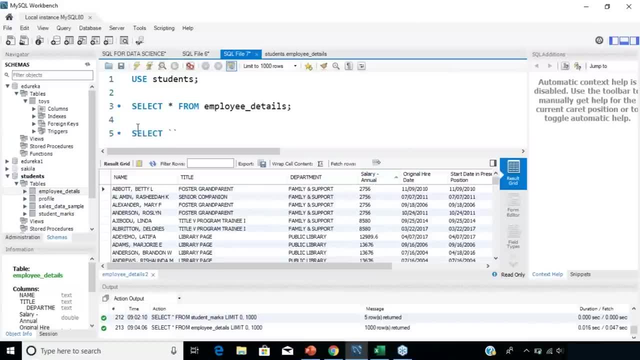 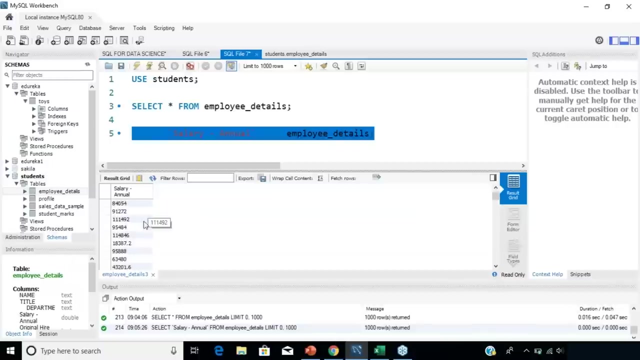 Okay, in our case it is salary annual right, So let's write that down- Salary annual right- from the name of your table employee details. Okay, so let's run this. So this query basically just gave me the salary column in my table, right, salary, and this is the salary. 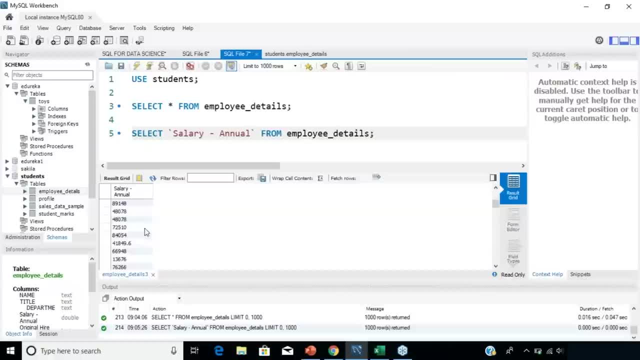 of all the employees that are there, And it's as simple as that. Now let's write a query to display the unique designations for the employees, basically unique job roles will display. So for that again, we have select because we're extracting. then 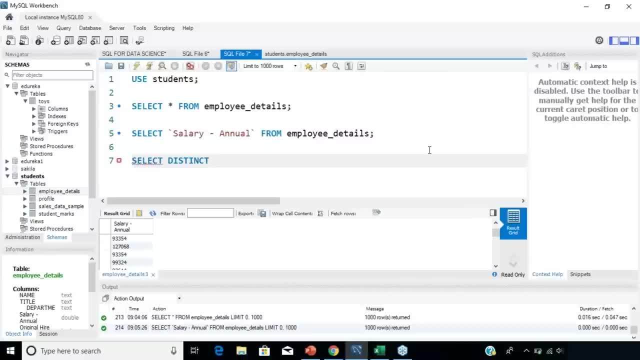 we have a keyword called distinct. since we are trying to display the unique designations, It'll just take the designations that are unique. It won't take your repetitive designations. For example, they might be 10 employees who are working as data analysts. 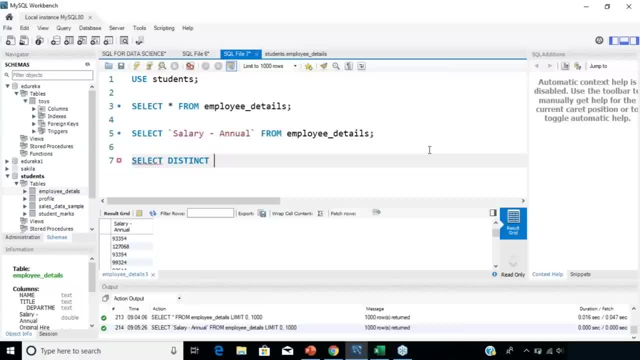 So we'll just consider that as one. So we're just extracting the unique designations for the employees. That's why we have the word distinct here. next, our job title is in the variable title. So that's why I've written title here and then we have from and the name of your table. 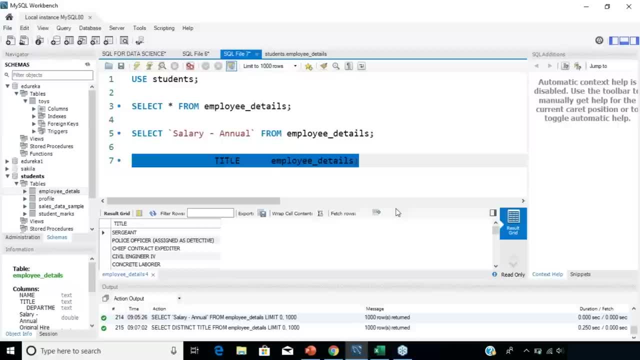 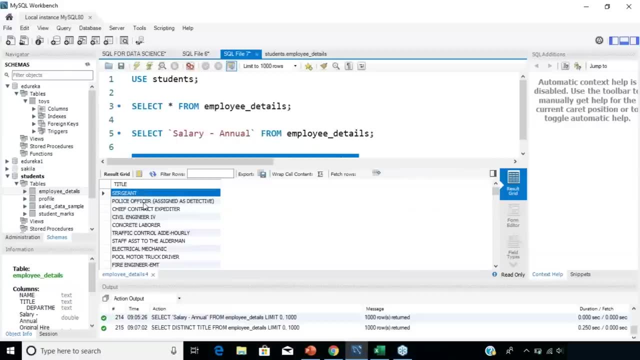 Right, Let's run this command. So here you can see that there are different job titles in our data set. We have surgeon, We have police officer, We have chief contractor, Expeditor, We have civil engineer, concrete laborer, We have traffic controller, pool motor. 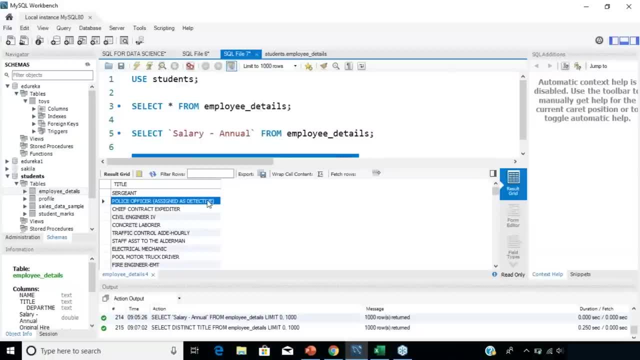 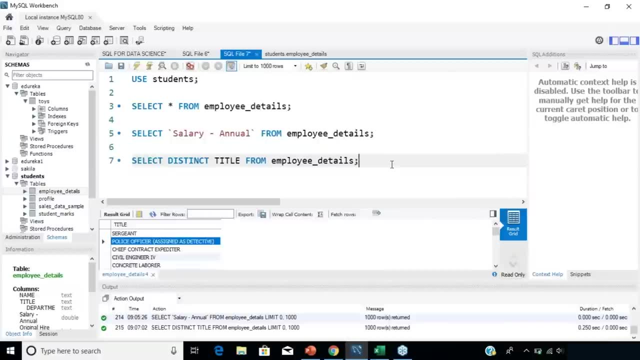 This is police officer and this is police officer assigned as detective. Wow, that's interesting, And so, basically, this query gave us the unique job roles that are there in our data set. Now let's try something else. Let's write a query. 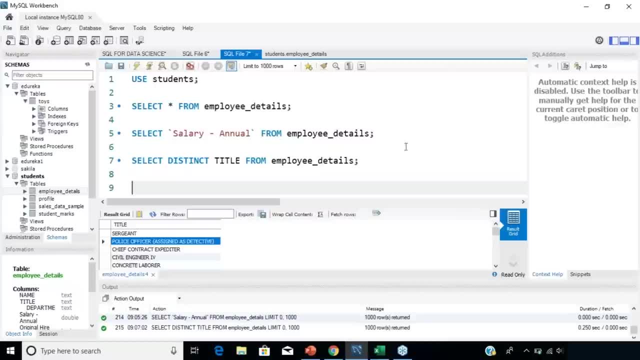 to display the unique departments with their jobs. So let's extract that. so select again. since we are trying the unique, we are going to use a distinct keyword and we are going to extract the unique departments and the job titles And from the name of the table. 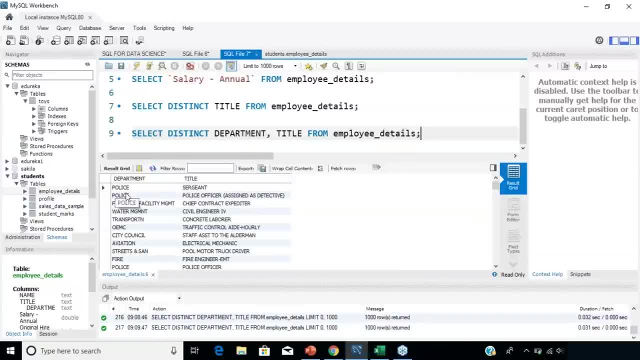 So let's run this code Now. under police department we have different job titles. That's why this is repeated here at we have police officer. Then there is fleet and facility management, under which we have a chief contractor as Expeditor under water management Department. 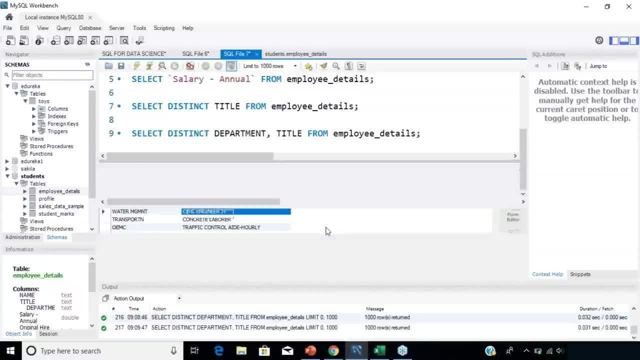 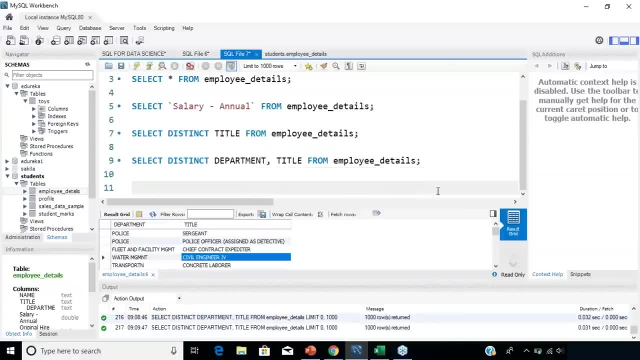 We have a civil engineer, and so on it. So, guys, this query was pretty simple. It just gave us the distinct departments according to their job titles. Now let's perform another query. will write a query to list the employees who are working in a particular Department. 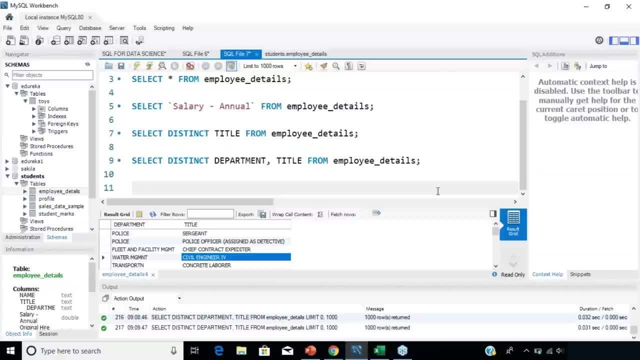 Let's say the fire Department. again, since we're extracting, we'll use the keyword select, after that select star from and the name of your table, Where. so this is where the where clause comes, and we're trying to identify a particular Department, So we'll put where department in the name. 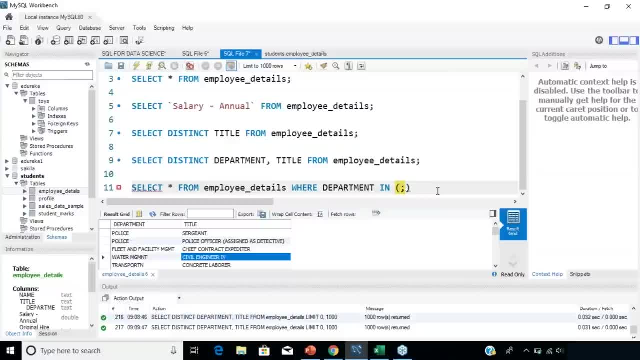 of the department that we're looking for, Let's say fire Department. that sounds interesting, So let's run this All right. So here you can see that we've just got employee details of all the employees that are there in the fire Department. 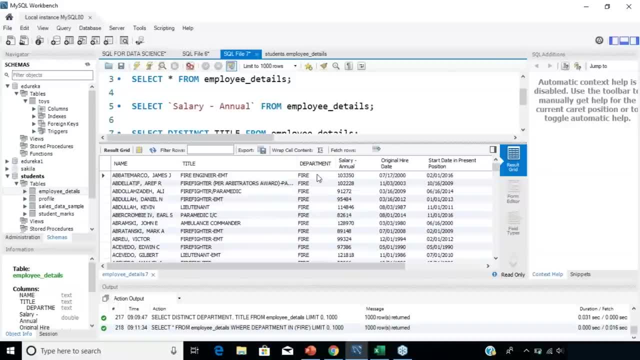 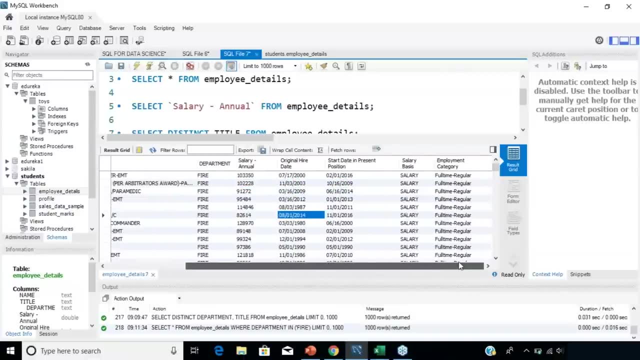 These are their salaries, These are the dates that they were hired on and, apart from that, this is the employment category: full-time, part-time. salary basis is whether you're getting paid. whether you're getting paid for the job. whether you're getting paid for the job. 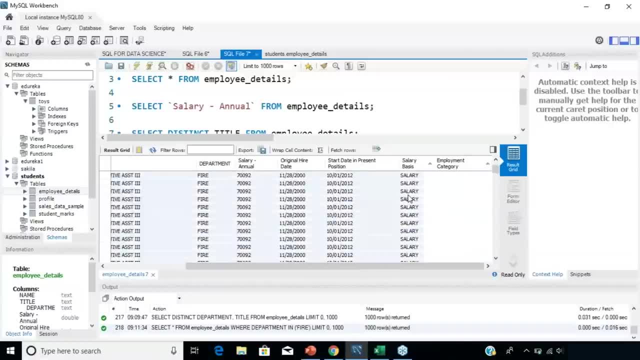 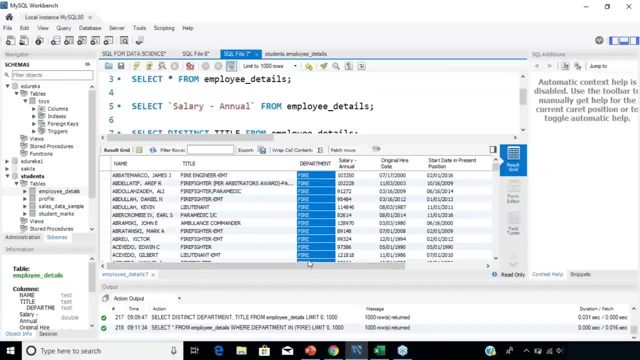 whether you're getting paid hourly or whether you're getting paid on a daily basis. So these are the details of all the employees that are working in the fire Department. If you see that here, it's entirely fire Department. So that was also quite simple. 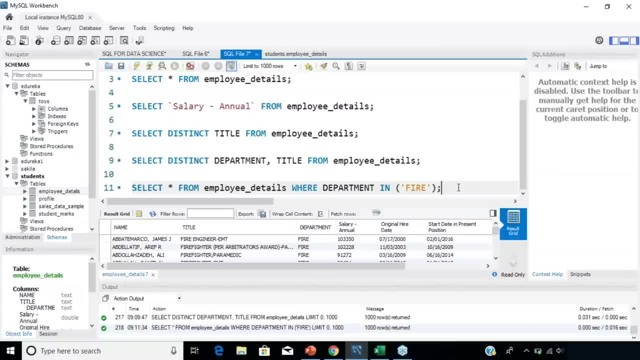 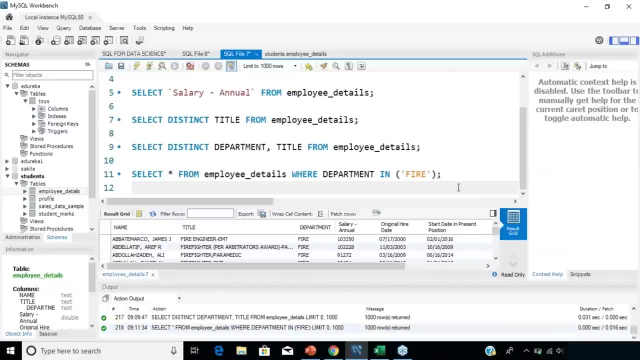 So this is how SQL is. The language is very, very simple because it's pretty understandable. like you can read the statement and you can understand what exactly I'm trying to extract or what exactly I'm trying to do. next Let's try to do something interesting. 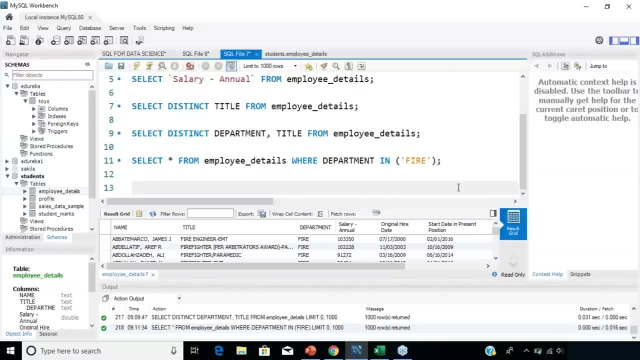 Let's say that we want to write a statement in the query to list the employees who do not belong to a particular Department. Let's say that we're trying to list out the employee details of employees which are not in the police Department. So for that it's quite similar to our previous query. 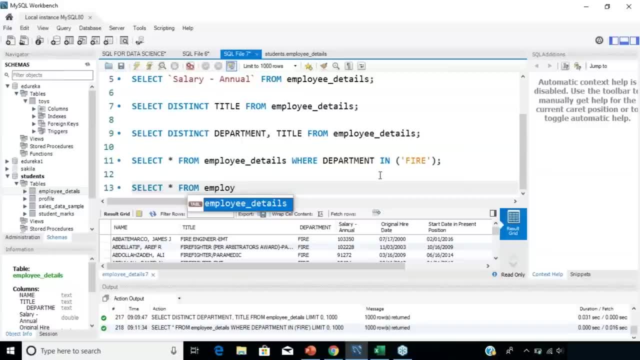 So you'll write select star from name of your table again, Where department not in. that's the only difference. Okay, not in, and the name of the department that you want to exclude. So this time let's say police Department. So we want only details of employees. 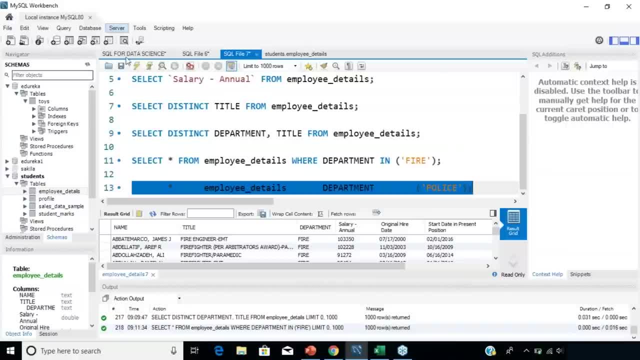 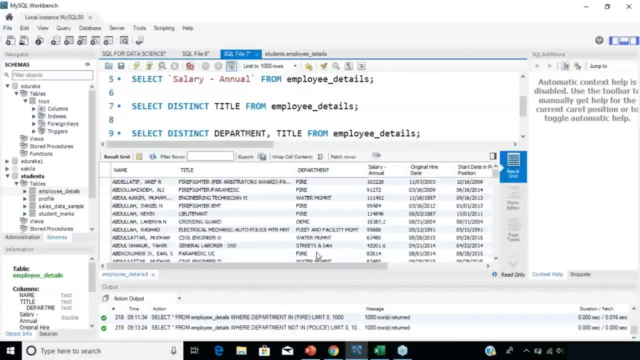 that are not there in the police Department. So let's run this, So all the departments here will have everything apart from your police Department. Okay, so we have fire, We have water management, We have law, We have streets and San, we have Finance Department. 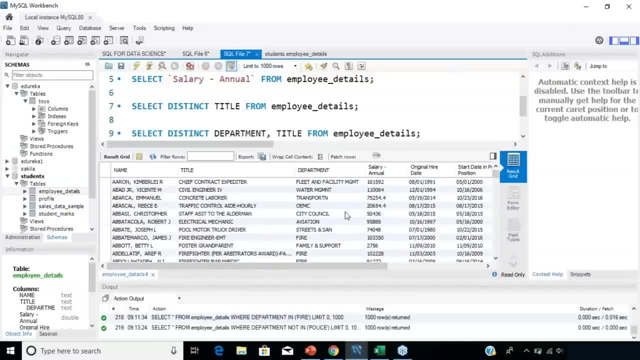 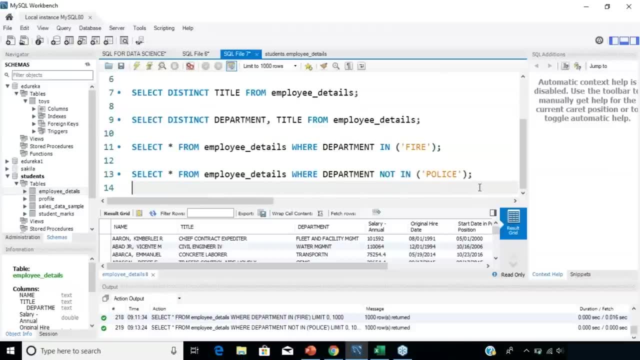 We have fleet and facility management and all of that. So, basically, we excluded our police Department and printed out the details of all the employees which are in every other Department apart from the police. All right, So now let's write a query to list the employees. 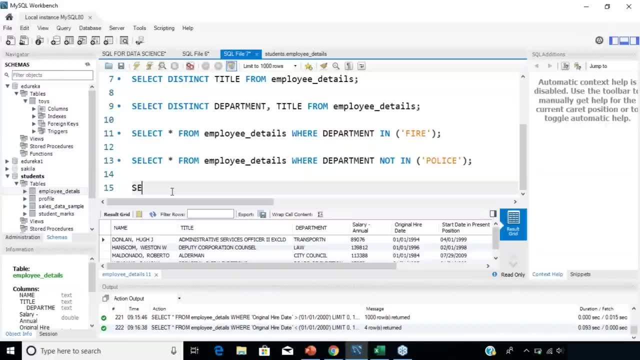 who joined before a particular date. So for that again we'll start from select star from name of your table right and we'll add the where clause, and here we'll mention our original hiring date, since that's the name of the variable that has the higher dates in it. 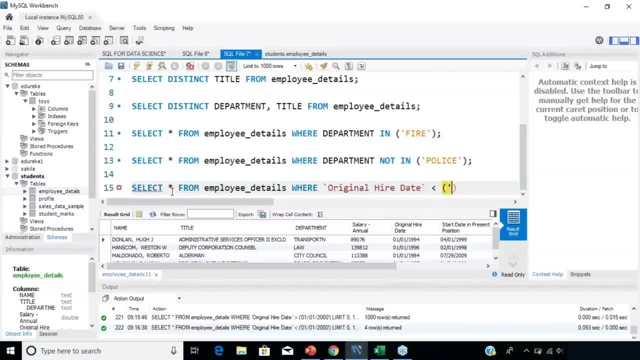 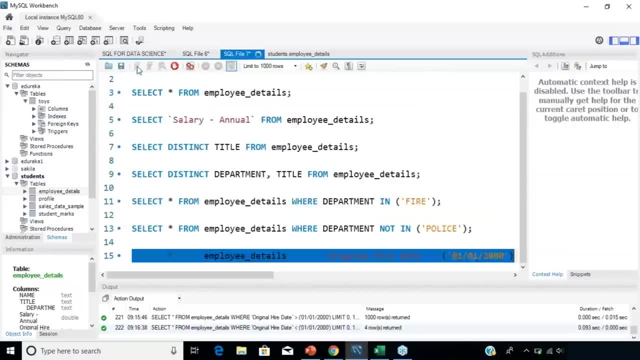 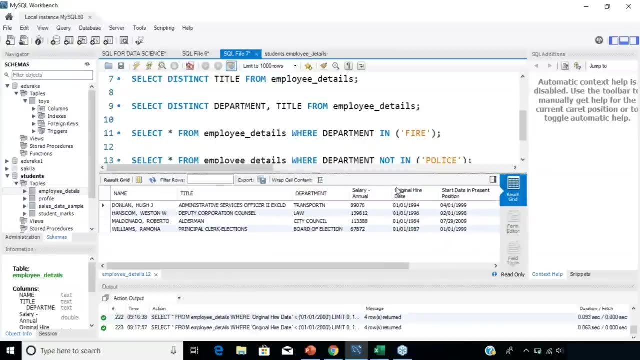 Let's keep it less than a particular date. Okay, let's choose first of January 2000.. Let's run this code. And so when you run this code, you'll find all the employees that were hired before 2000.. So if you see original hire date, 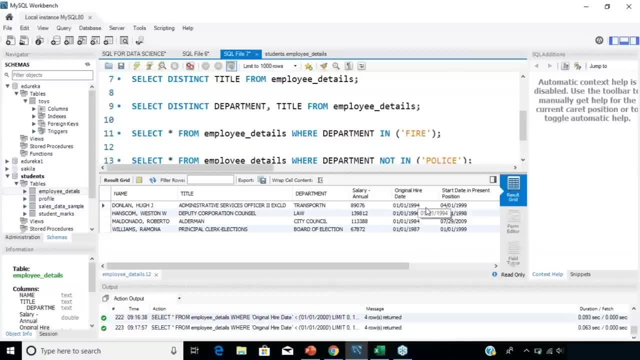 all of this is before 2000.. Some of them were in 1994, 1996, 1984 and 1987. So the only four employees who are hired before the year 2000, basically before the first of January 2000.. 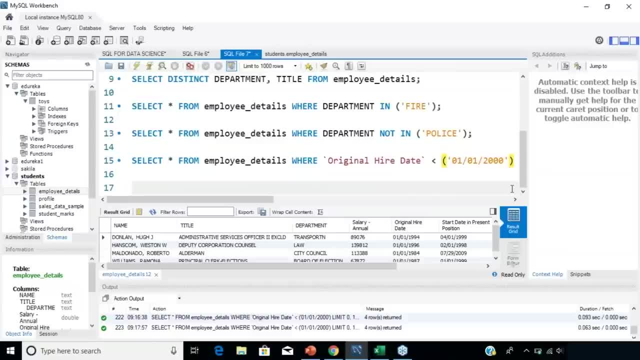 Now let's try another query. Let's write a query that will display the average salaries of all the employees who work at a particular Department. Okay, let's choose the surgeon Department. So, basically, we're going to display the average salaries of all the employees who are working as surgeons. 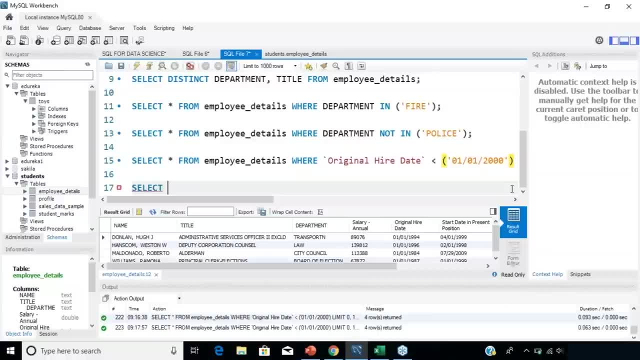 So for that again, it starts from select. since we have to calculate the average salaries, We'll use a function called average, which is a predefined function in sequel, and average of which column it is a salary column, salary Annual, and let's mention the name. 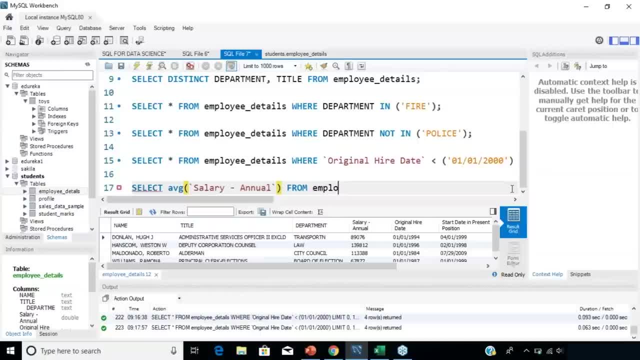 of the table from employee detail Some error. Let's write down the whole statement and then we'll see what the error is. So we're going to do this and we're going to select the job title as a surgeon, Basically the average salary of a surgeon. 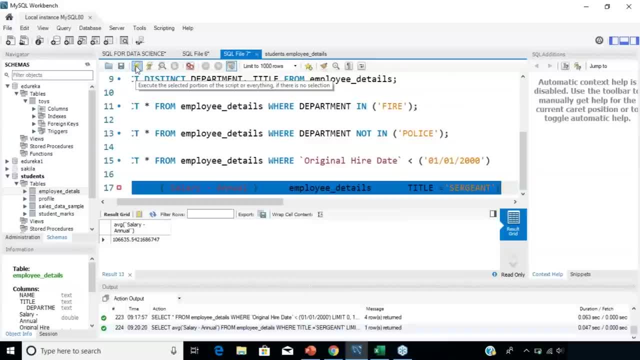 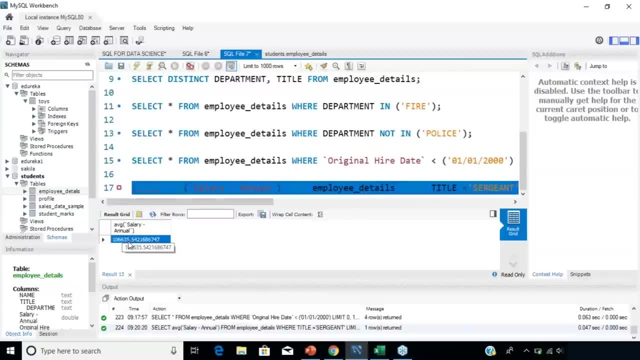 Let's run this first and we'll find out what the error is. Okay, there is no error. I have no idea why I'm getting this. So the average salary is around one lakh six thousand, and change right for a surgeon. So now let's try another query. 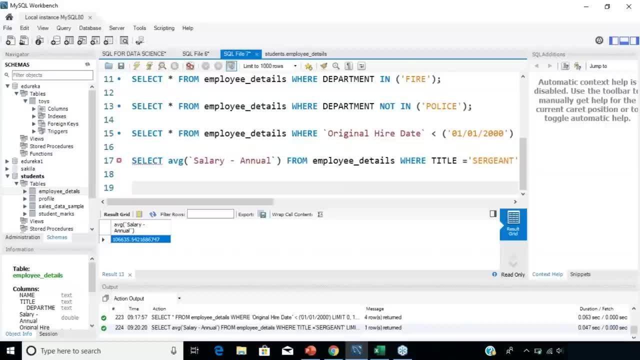 What we can do is we'll write a query to display the details of a particular employee. Some name will select at random. Okay, So select star from name of your table. employee details where name is equal to. let's look for a particular name. 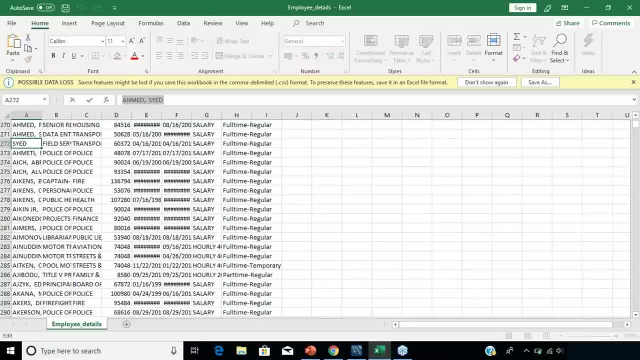 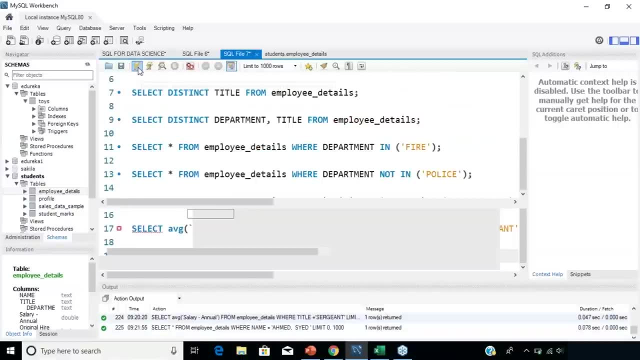 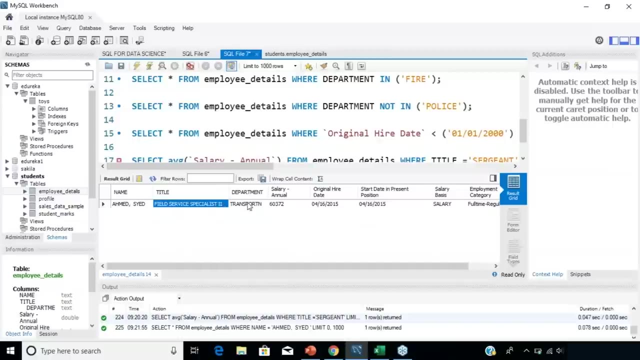 Ahmad Syed. Okay, So name of the employee. Let's paste that name over here, right? Hopefully they should give us an output. Let's run this. So now we have the details of this particular employee, who is Ahmad Syed, his title, job title, his department. 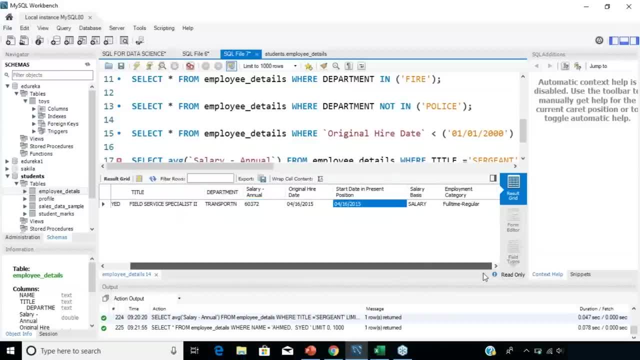 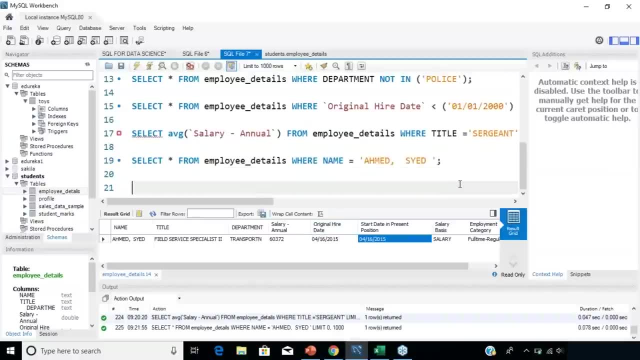 his salary, all the details about him. So we just printed all the details about a particular employee. Now let's try something else. Let's write a query to list the employees whose salary is, let's say, more than 3000.. After giving a 25% increment to their salary, 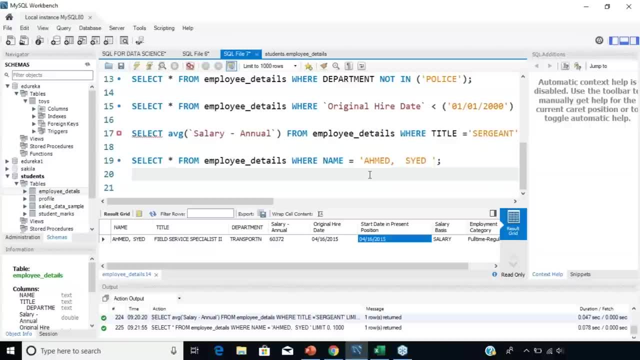 Now let's do a little bit of math. So we list down employees whose salary is more than 3000, after giving them a 25% increment. So let's write down a query for that. So again, start off with select star from the name of your table. 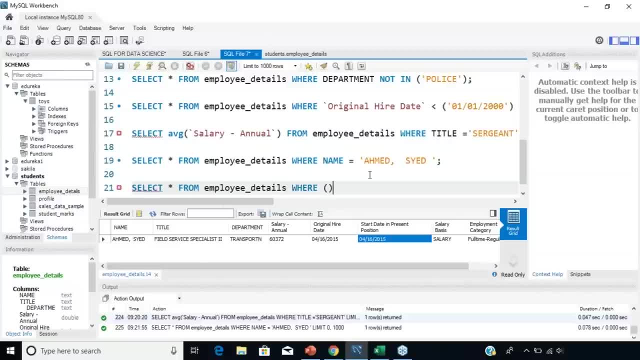 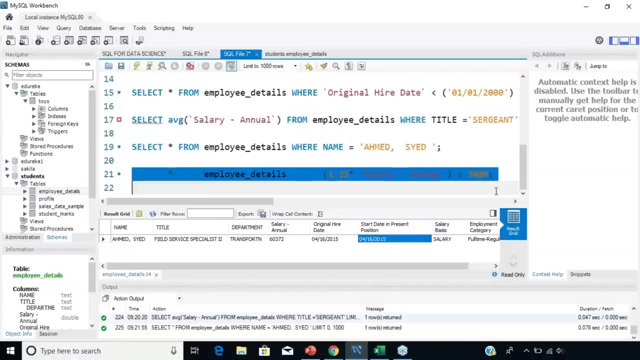 where? here will specify the condition: basically, after giving them a 25% increment- 1.25 into the salary, So salary annual- and after giving them a 25% increment, their salary should be at least 3000.. All right, So this is exactly what we're doing here. 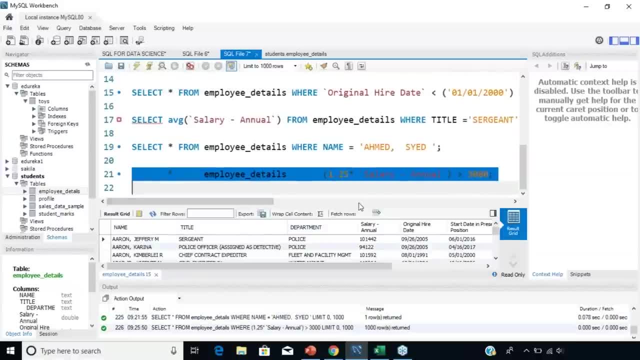 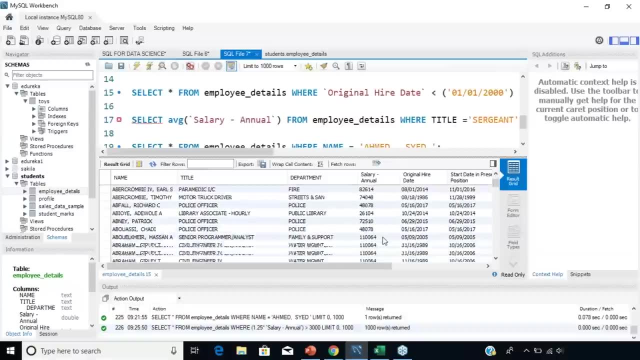 Let's run this code and let's see if we're getting anything. So here are the employees whose salary is more than $3,000, after giving them a 25% raise. So basically, these guys are promoted. This is a list of all the employees. 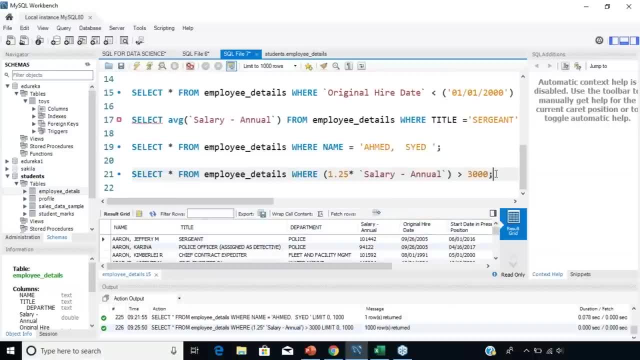 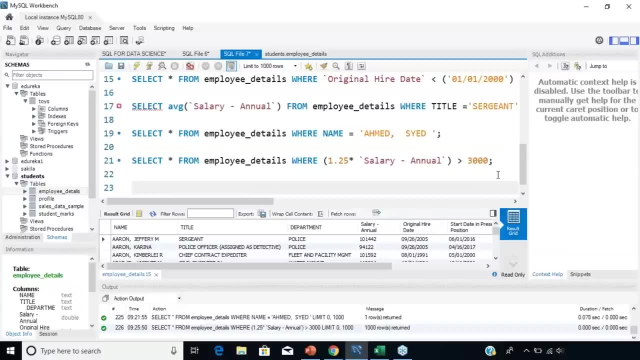 So that's quite simple, guys. It's basic math implemented in one line of code. That's how simple SQL is. a lot of data scientists require this kind of tool, because querying even your complicated math and even complicated things from your database becomes very easy when you make use of SQL languages. 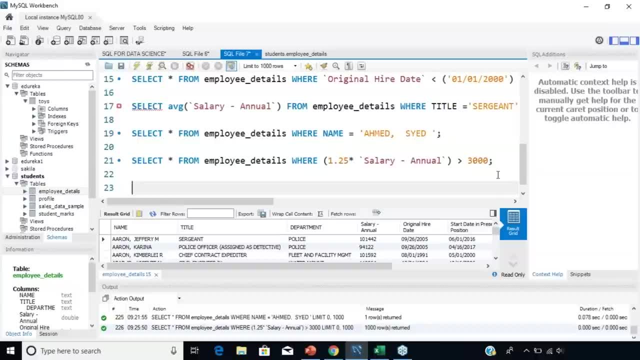 it becomes extremely easy to even do the complex things. Now, I just did this in one line, So now let's try something else. Let's write a query to list the employees whose salary is less than a particular number. Okay, let's say less than $3,500. 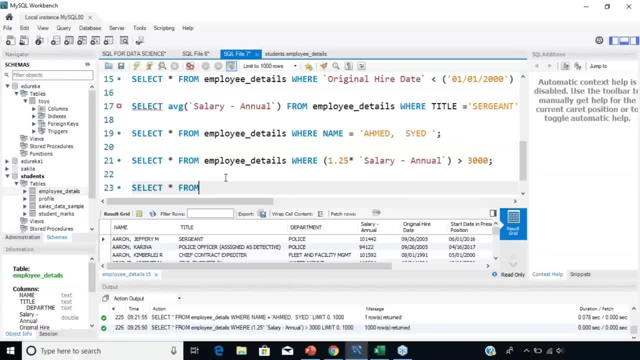 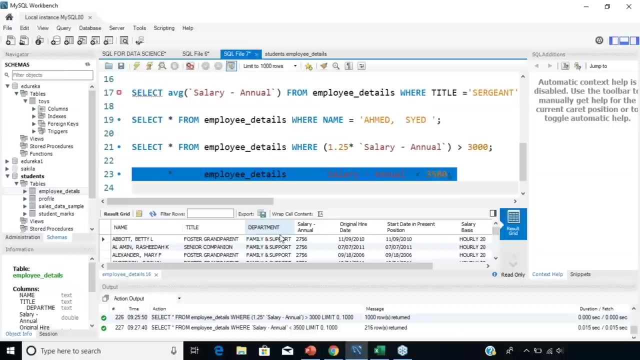 So let's write a query, basically for employees whose salary is less than 3000 or 3500. Where salary annual is less than, let's say, 3500. So let's run this line of code. All right, so we have a couple of people. 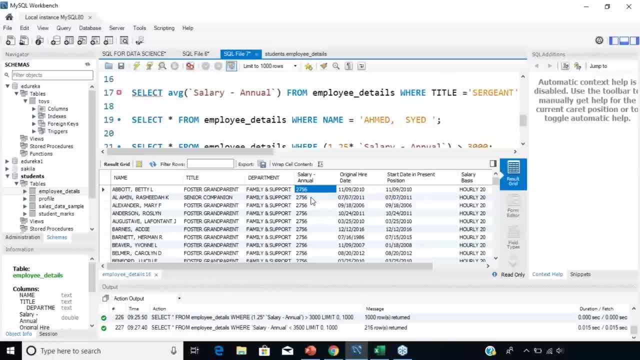 whose salary is less than 3000.. So we have 2756 like maximum of these people have 2756.. Okay so, basically this is a list of employees whose annual salary is less than $3,000.. That's also quite simple to do. 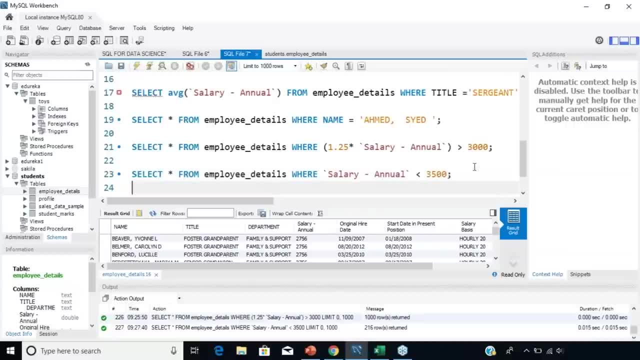 It's just one line of code. Now let's try something else. We'll write a query to list the names and a particular set of deals about an employee who joined before a particular date. Let me write it down for you, and then we'll understand what exactly I'm doing. 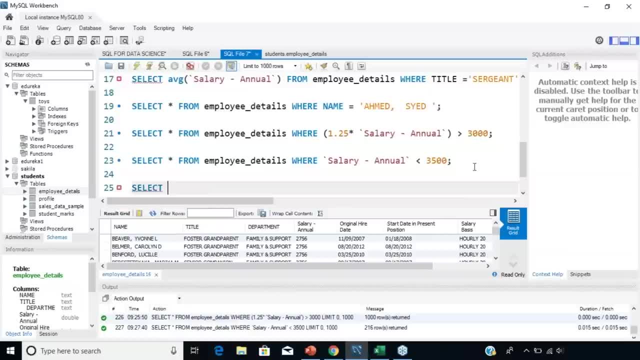 So select. now we'll define a variable so that we can basically extract a number of columns. Okay, So let me write this down and then I'll tell you what exactly I did here. name: and let's also get their salary right. original Hiring date. 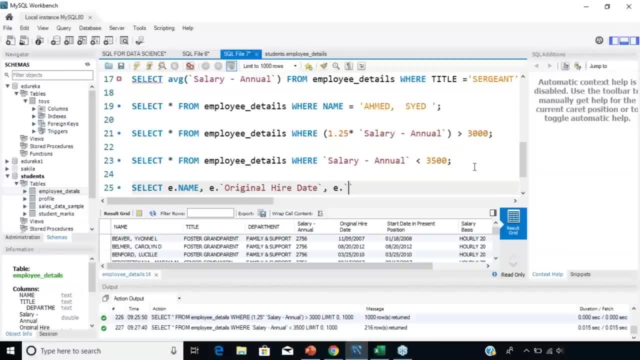 Then we'll also get the salary From the name of the table Where the hiring date- Let's say it was lesser than, and give a random number- 0102, 2008.. Now, what exactly I'm doing here is I'm basically listing out the name of the employee. 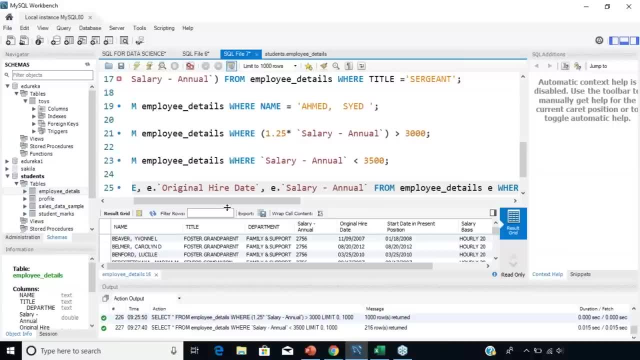 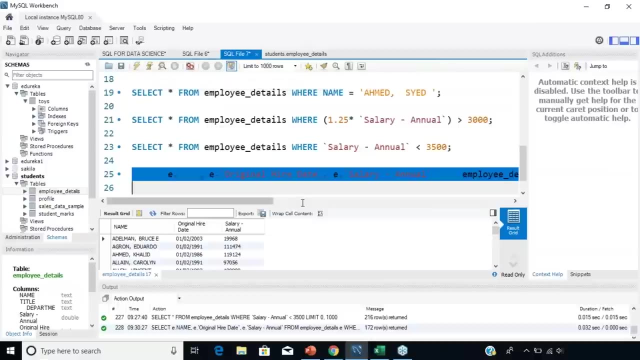 the hiring date and the salary of all the employees that have joined before a particular date. Okay, basically before this date. That's what I've done here. Let's run this line of code and let's see if it works Right. So here we have the name, the hiring date, 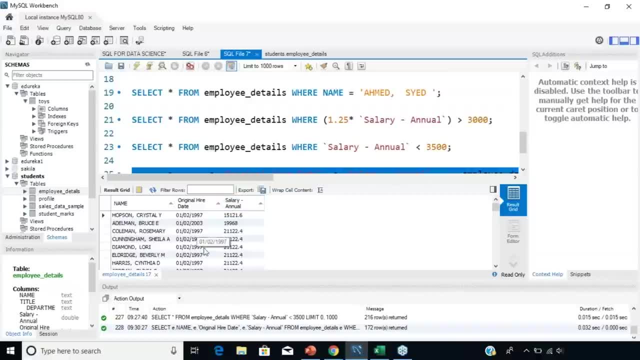 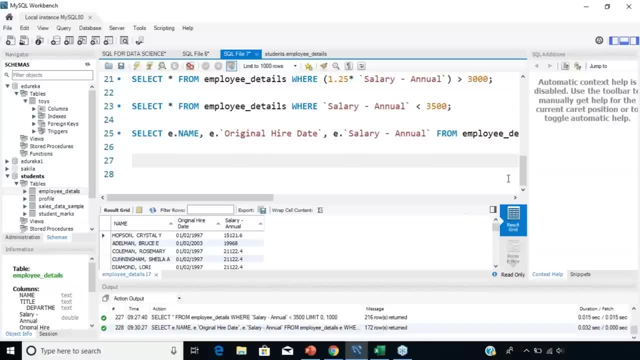 and the salary of individuals that have joined before a particular date in 2008.. So it's as simple as that. Now let's write a query in SQL to list all the employees who joined on a particular date. Okay, Let's say we want the details of all the employees. 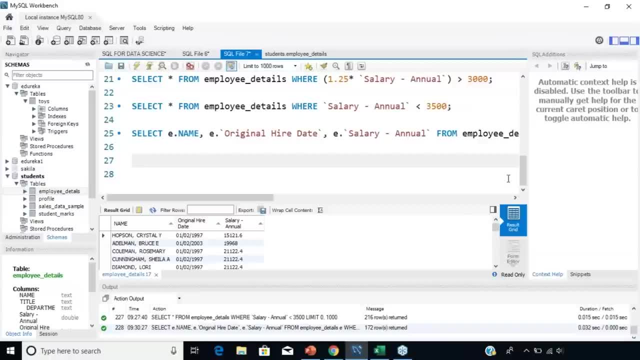 who joined on October of 2013 or something like that. for that again, It starts off with select star from the name of the table. We'll add the where clause along with the hiring date: Original hire date, a particular date, Let's say 0, 8 2013.. 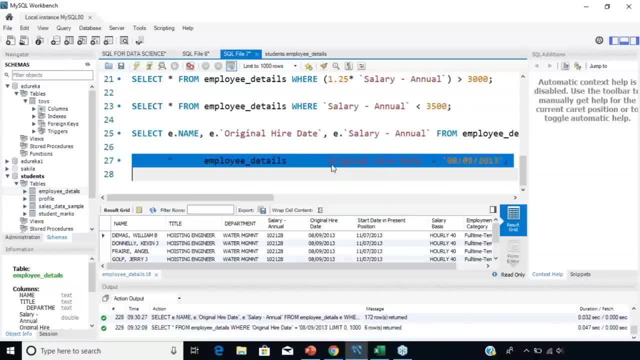 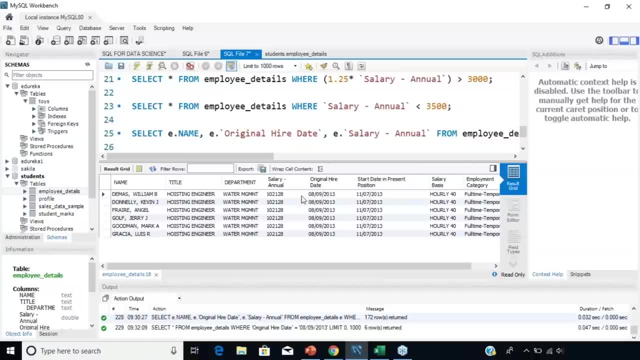 Let's run this line of code. So, basically, we list down employees that were hired on this particular date. Okay, these are details of all the employees that were hired on the same day. So we have around six employees that were hired on the 8th of 2013- some date. 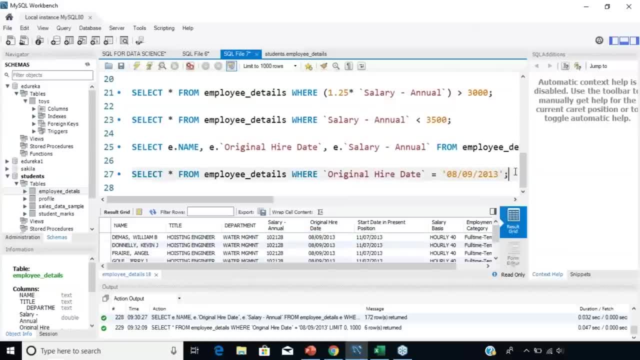 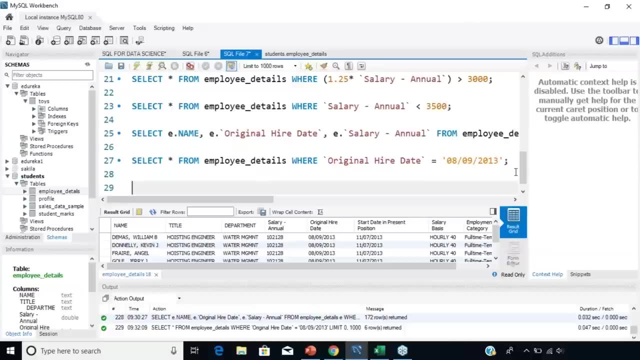 Okay, Right. So, guys, that's what you see. SQL is a very easy language. You just have to understand what you're trying to extract. That's all you just have to know like 5 to 10 basic commands, and these basic commands can do wonders. 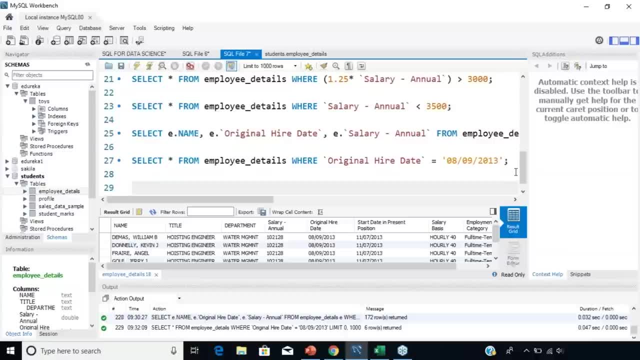 They can extract and manipulate data in such a way that you know you can perform proper data analysis, data processing and so on. Now let's try one last query. Let's write a query to list the employees whose annual salary is within a particular range. 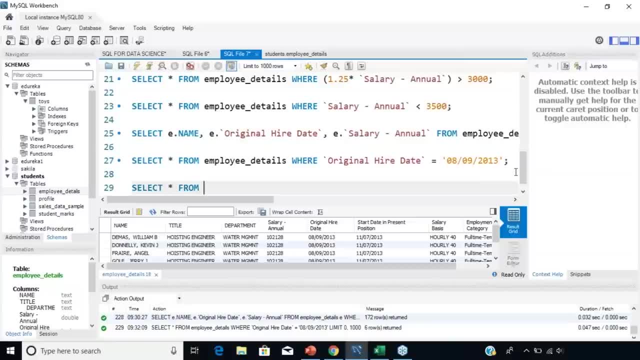 for this again, We have select star from name of the table, Employee details, and let's add the where clause and here we will say: salary Annual is between, between, as another keyboard, So between two numbers, okay, let's say between. on $24,000: 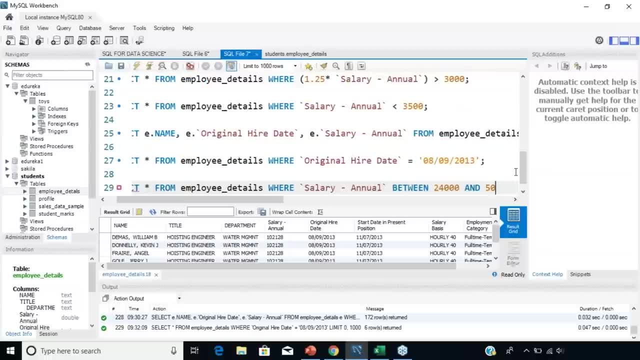 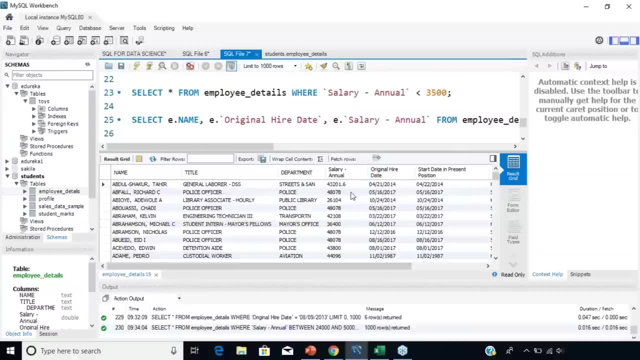 and let's say 50,000.. Right, Let's run this line of code, All right. So here you can see that all of these employees have a salary range between 25,000 and 50,000.. So 43,201, we have 42,000.. 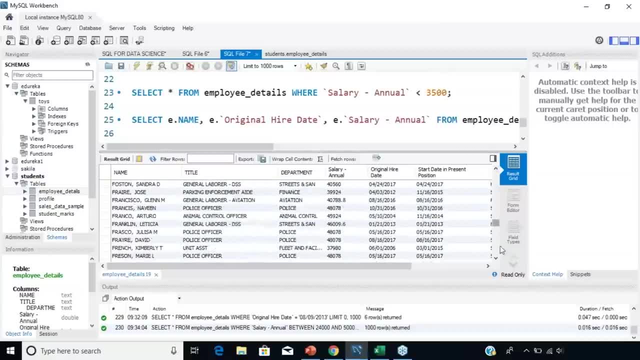 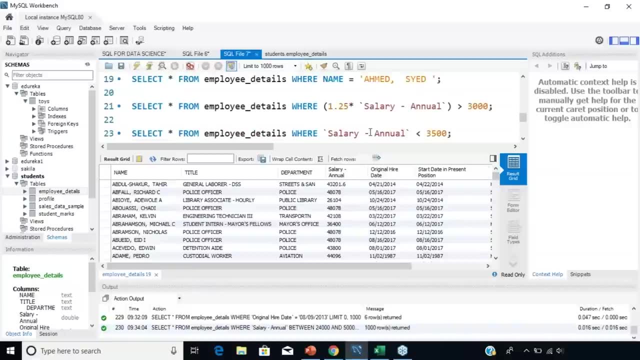 You have 44,000.. We have 45,000. 48,000 as a maximum salary, All right, So this is basically how you perform querying using SQL. So if you're an aspiring data scientist and you want to become a professional data scientist, you need to make sure that you are skilled with SQL. SQL is one of the most important querying languages that you need to know in order to become a data scientist. You look at any job description. You look at any company that's hiring a data scientist. 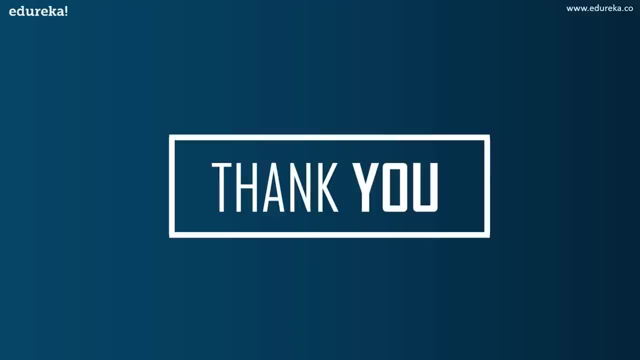 There will always be a prerequisite: that you have to know SQL. and, guys, SQL is not difficult at all. It's a very easy language. It consists of a set of, let's say, 20 to 50 commands, Max to Max, and you just have to know. 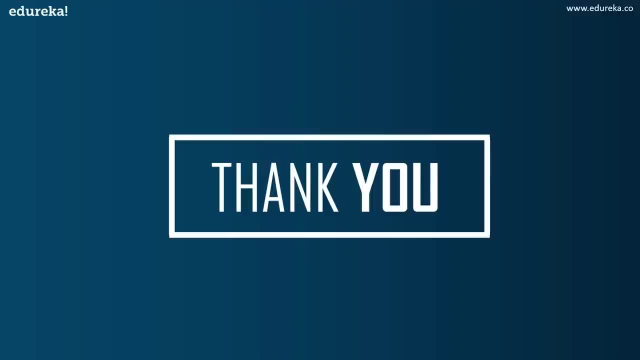 how to play with these commands in order to derive useful insight from your data. So that's all from my side for this session. If you have any doubts, please let me know in the comment section. until next time, happy learning. I hope you have enjoyed listening to this video. 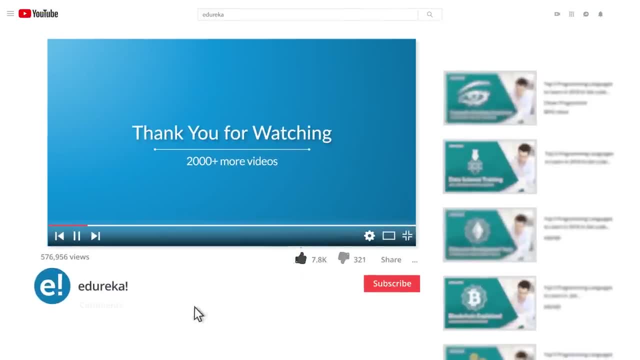 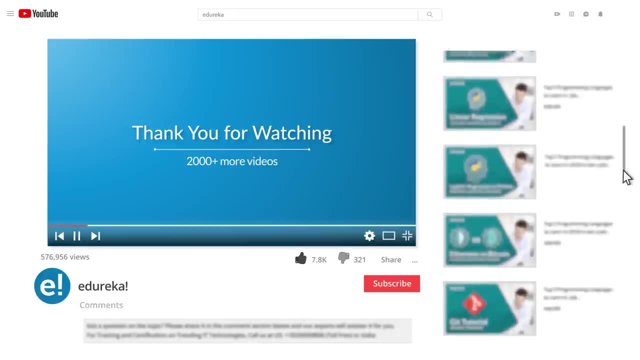 Please be kind enough to like it and you can comment any of your doubts and queries and we will reply them at the earliest. Do look out for more videos in our playlist and subscribe to Edureka channel to learn more. Happy learning.